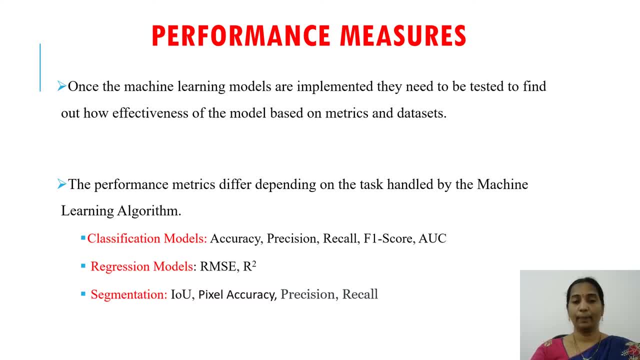 or the affected region. So appropriate measures are IOU- IOU stands for intersection over union- Or we can even use pixel accuracy precision Recall also. So in this talk we will confine to the accuracy of the classification models. So let us see in detail what are the different measures that can be used on the classification. 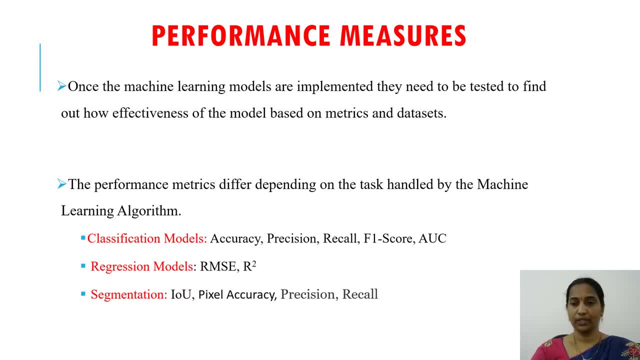 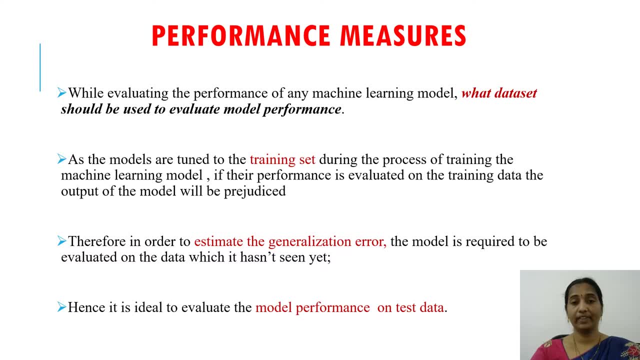 models and when to use which measure. Once the model is available, then its performance has to be evaluated. Then the question is on what data the performance of the model has to be evaluated. So we can evaluate the performance of the model on the training data. 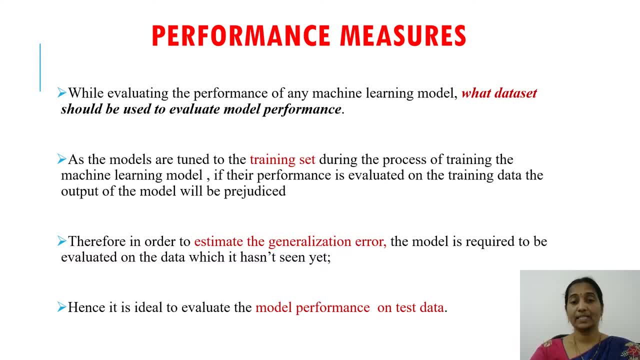 itself. But the problem here is when the model is tested using the training data, the results will be biased towards the training data because the model is already tuned to the training data. So the output of the model would be anyhow good on the training data. So that is why measuring the 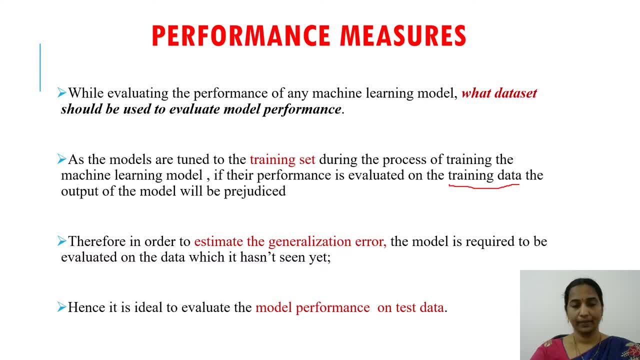 performance of a model on training data is very important, So let us see in detail what are the model's performance on a given playing fieldここ l affects data performance on data with бел目age t, due to which the America model has never had more performance than this model. 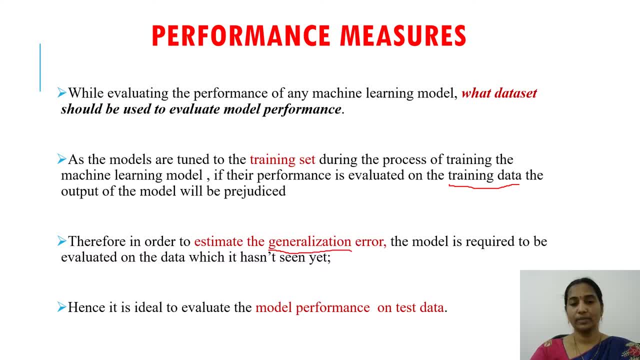 per se, So you can simply count these numbers from each generation. If it is because of N sample or because the model had very little performance, that means that the model has very small performance and the model has a high performance level. in this cases, only controlling. 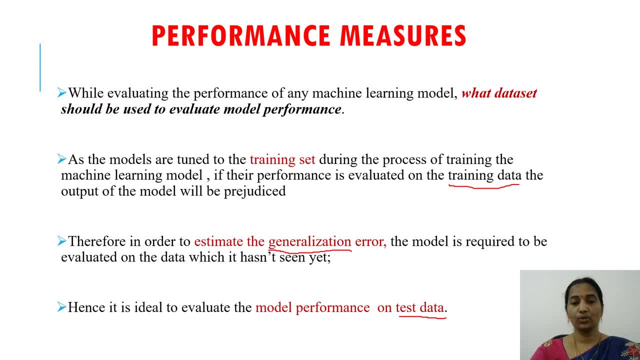 on. So test data is a set of examples which is not shown to the model during its training. So the ideal case is evaluate the performance of the model on the test data and use it as an indicator to show the effectiveness of the model. 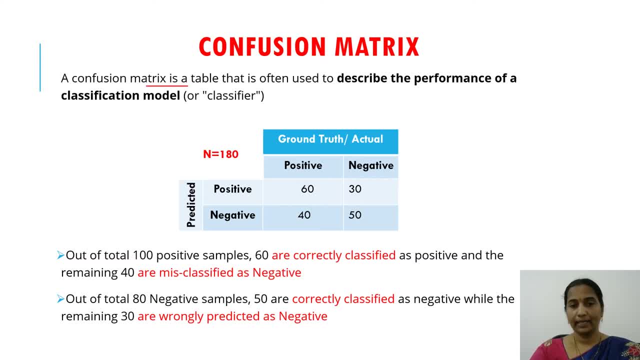 So confusion matrix is basically a table that is often used to understand the performance of any model, So a classifier. basically, This is a sample of the confusion matrix for a given model. Model is evaluated on 180 samples, So n means the total number of samples and the ground truth means the actual data. 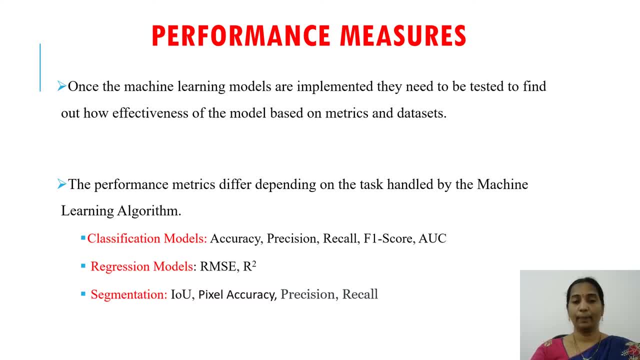 or the affected region. So appropriate measures are IOU- IOU stands for intersection over union- Or we can even use pixel accuracy precision Recall also. So in this talk we will confine to the accuracy of the classification models. So let us see in detail what are the different measures that can be used on the classification. 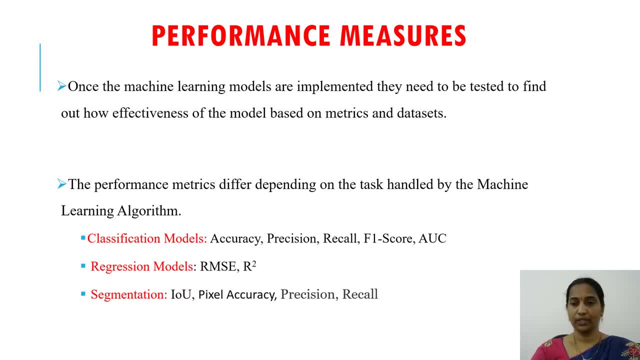 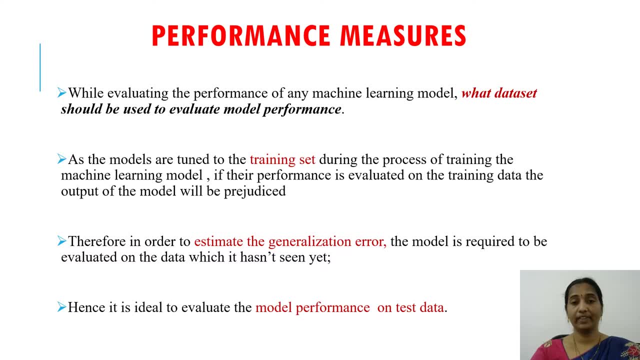 models and when to use which measure. Once the model is available, then its performance has to be evaluated. Then the question is on what data the performance of the model has to be evaluated. So we can evaluate the performance of the model on the training data. 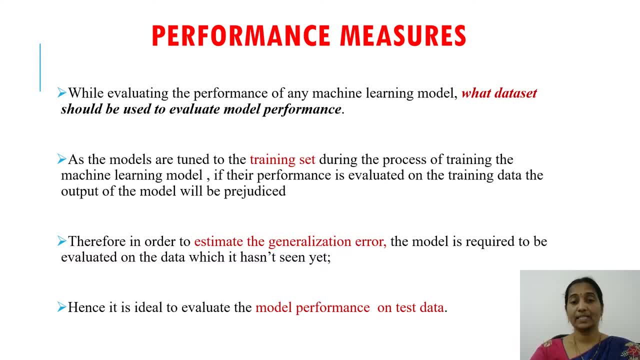 itself. But the problem here is when the model is tested using the training data, the results will be biased towards the training data because the model is already tuned to the training data. So the output of the model would be anyhow good on the training data. So that is why measuring the 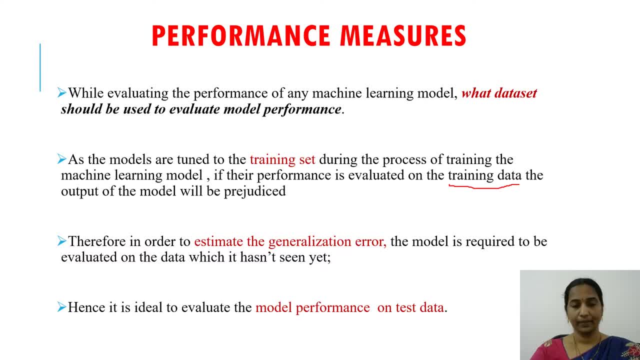 performance of a model on training data is very important. So let us see in detail what are the different measures that could be used To better understand the overall generalization ability of the model. there is information first about its performance in the training, So we can taking 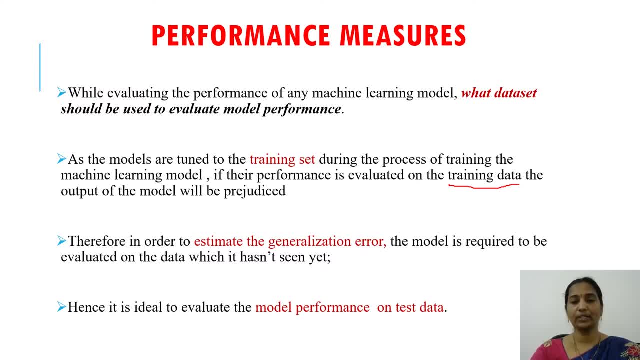 advantage of the generalization ability we used earlier, given we said that application and it is not visualize in the model before and then we put into a model model. we have some data and evaluation data, So to better understand the generalization ability of a model we have to 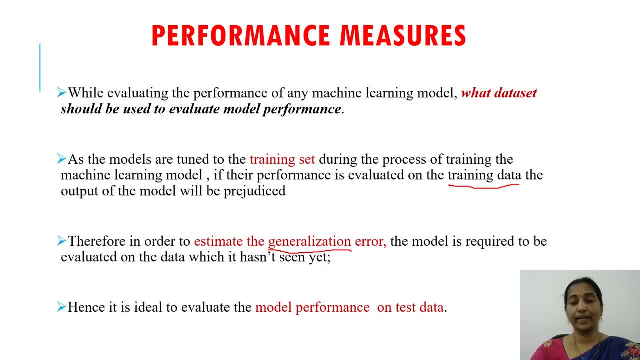 use some other data to understand therun the model without being seen by the model In generalization. So the generalization ability of a model means how well the model performs on the data that is not seen during the training To understand is generalizatit ability. we have to test its. 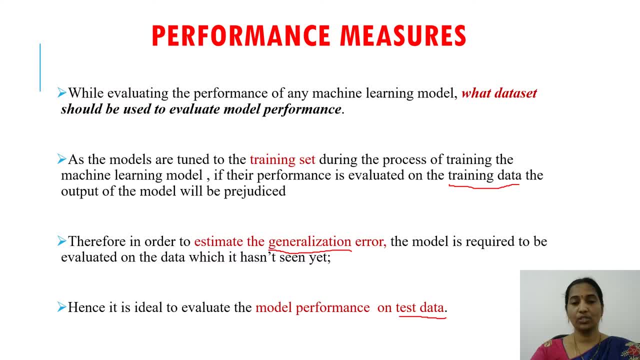 performance on the data called as test data. So this is for the new model model. We would have to. We would need to test the model before and after Recently models, design cases and data points and then we take a. So test data is a set of examples which is not shown to the model during its training. 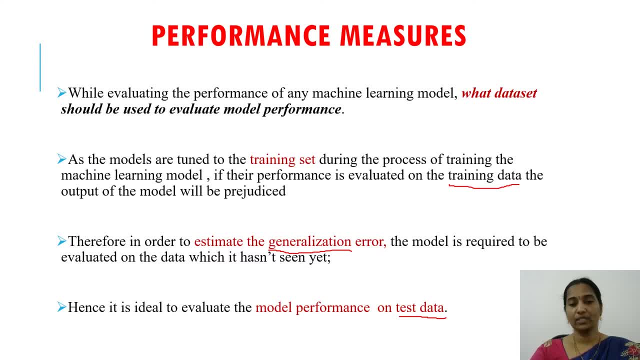 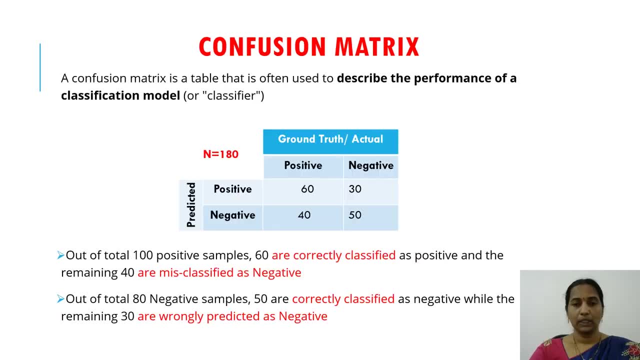 So the ideal case is evaluate the performance of the model on the test data and use it as an indicator to show the effectiveness of the model. So confusion matrix is basically a table that is often used to understand the performance of any model, So a classifier, basically. 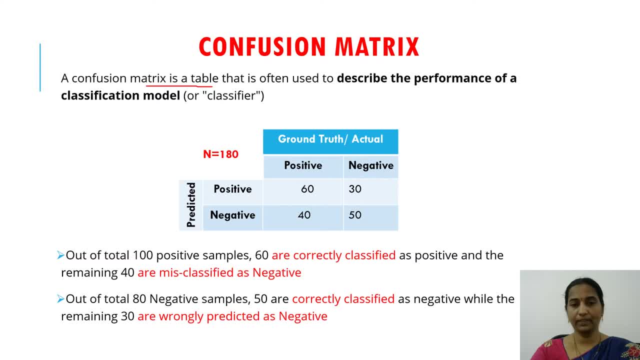 This is a sample of the confusion matrix for a given model. Model is evaluated on 180 samples, So n means the total number of samples and the ground truth means the actual data. So this is a confusion matrix taken for the binary classification task. 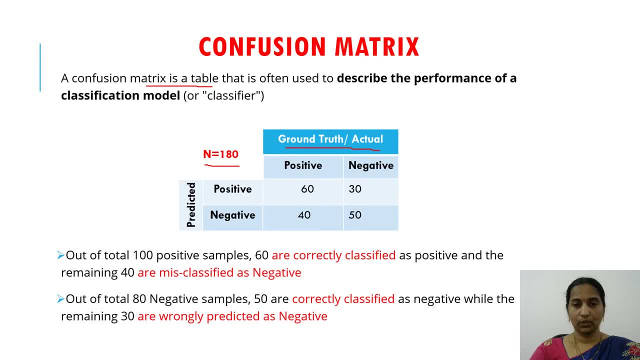 That is, we have two classes for the task. So we are considering the classes as positive and negative. In the ground truth case We have positive examples as 100, 100 positive, 100 examples under the positive class and 80 examples are the negative under the negative class. 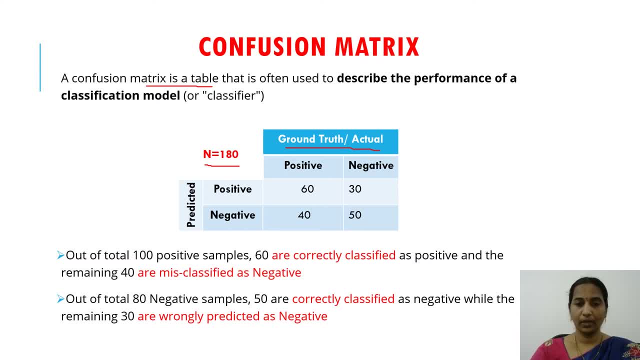 So each column indicates the class. So this is the positive class, this is the negative class, and so the column wise, when we observe it, indicates the ground truth of the data, and similarly, when we observe the values on the row wise. So here, if we observe this, 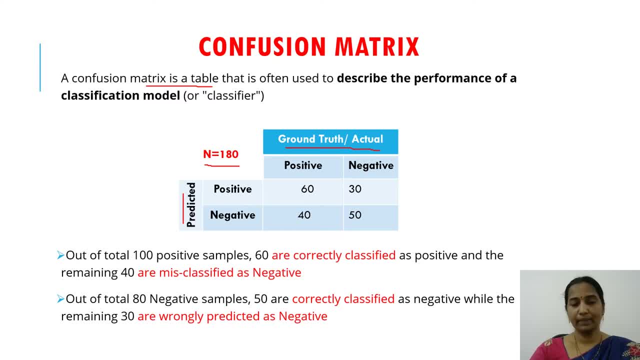 So this is the. So this is the predicted data. So this is that means the predictions, how the model is predicted. so that is indicated using the rows. So here also, as we have two classes, so we have two rows in the confusion matrix one. 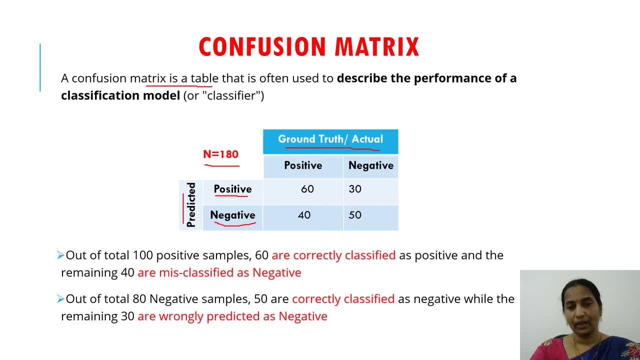 is a positive class and the other one is a negative class, and each row So how many examples are classified as positive by the model is we can under. we can get that value by summing up the row values of the across the positive class. 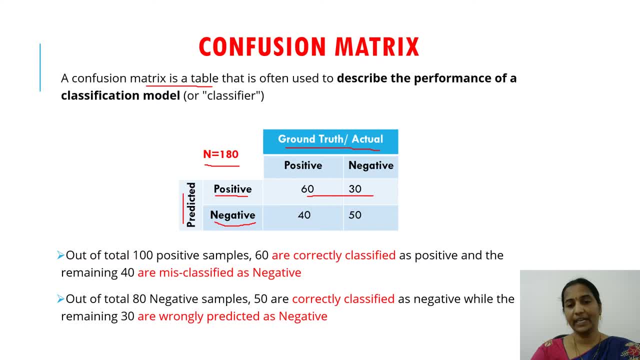 So 60 plus 30, that means 90, 90 examples are actually predicted as positive by the model. So that is what is indicated by each row of the confusion matrix and similarly, the second row indicates the how many examples are predicted as negative by the model. 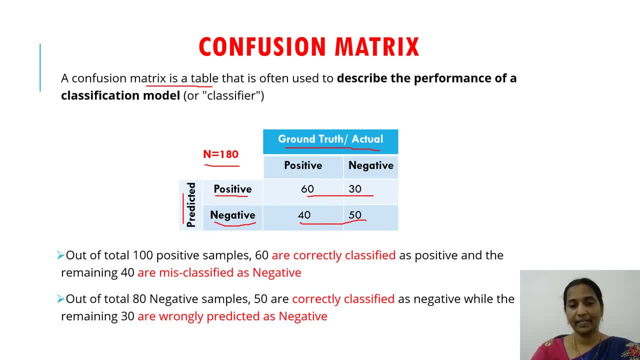 So in this case, so again, 90 examples are predicted as negative by the model. So, then, how to understand, how to use this tool to understand how many examples are predicted as negative by the model? So the effectiveness of the or the as a measure of the performance is here this, this: 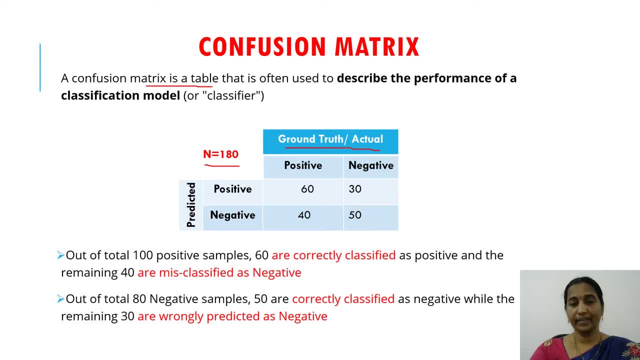 So this is a confusion matrix taken for the binary classification task, That is, we have two classes for the task. So we are considering the classes as positive and negative. In the ground truth case We have positive examples as 100, 100 positive, 100 examples under the positive class and 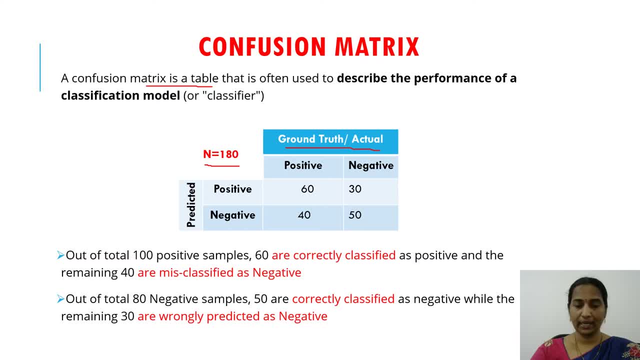 80 examples are the negative under the negative class. So each column indicates the class. So this is the positive class, this is the negative class and so the column, wise, when we observe it, indicates the ground truth of the data. and similarly, when we observe the 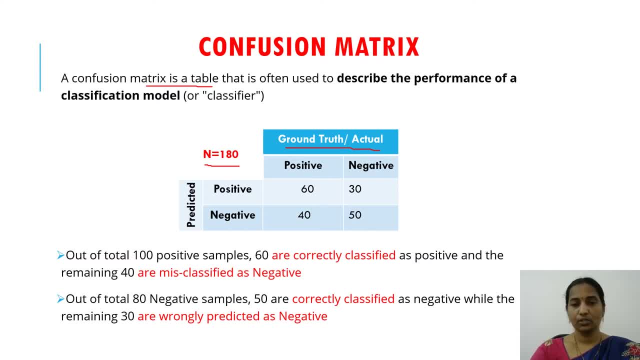 values on the row wise. So here, if we observe this, So this is the, So this is the predicted data. So this is that means the predictions, how the model is predicted. so that is indicated using the rows. So here also, as we have two classes, so we have two rows in the confusion matrix one. 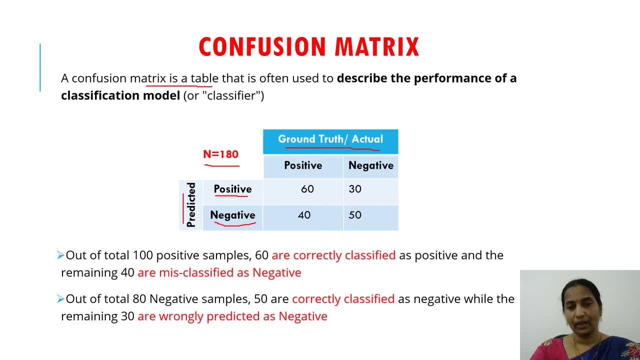 is a positive class and the other one is a negative class, and each row So how many examples are classified as positive by the model is we can under. we can get that value by summing up the row values of the across the positive class. 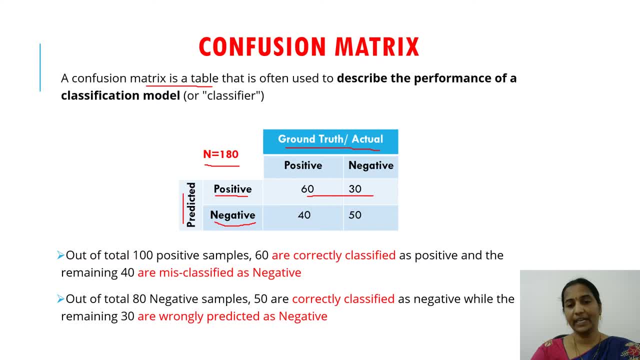 So 60 plus 30, that means 90, 90 examples are actually predicted as positive by the model. So that is what is indicated by each row of the confusion matrix and similarly, the second row indicates the how many examples are predicted as negative by the model. 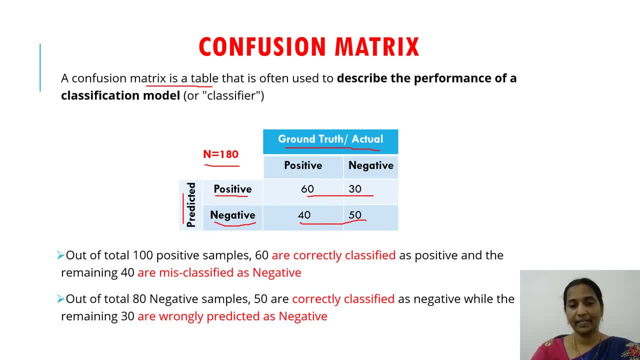 So in this case, so again, 90 examples are predicted as negative by the model. So, then, how to understand, how to use this tool to understand how many examples are predicted as negative by the model? So the effectiveness of the or the as a measure of the performance is here this, this: 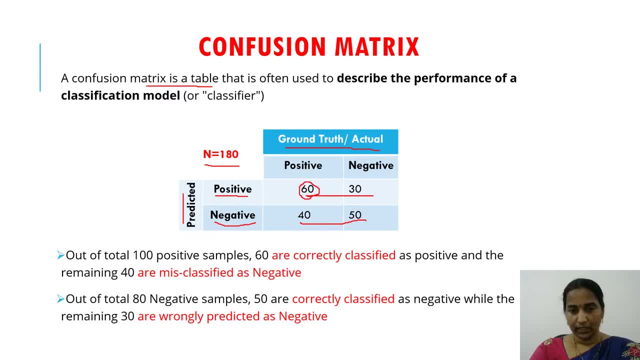 indicates. each cell indicates a measure So like. so this cell indicates how many of the examples are positive example. actually they are belonging to the positive examples 60 and they are predicted as positive. that means positive examples. original positive examples are predicted as positive. that means: 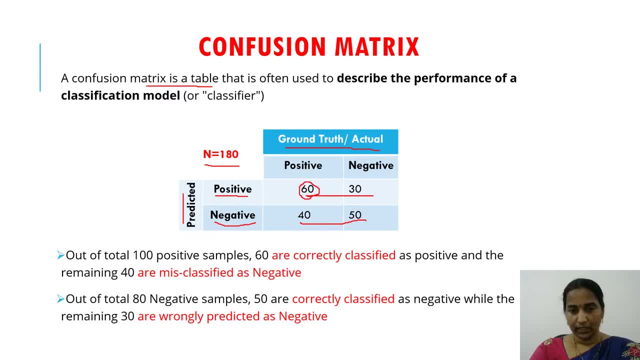 indicates. each cell indicates a measure So like. so this cell indicates how many of the examples are positive example. actually they are belonging to the positive examples 60 and they are predicted as positive. that means positive examples. original positive examples are predicted as positive. that means: 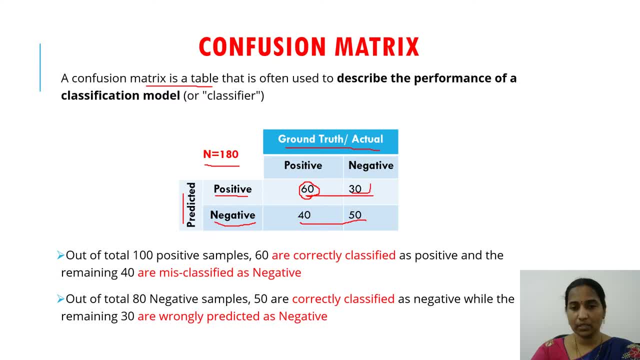 they are correctly classified. and here, if we observe this cell, the data in this cell, this indicates that actually these samples, these 30 samples, are belonging to the negative class, but they are by mistake predicted as positive by the predictor, by the model, So they are wrongly classified. that means these are wrongly classified, whereas these: 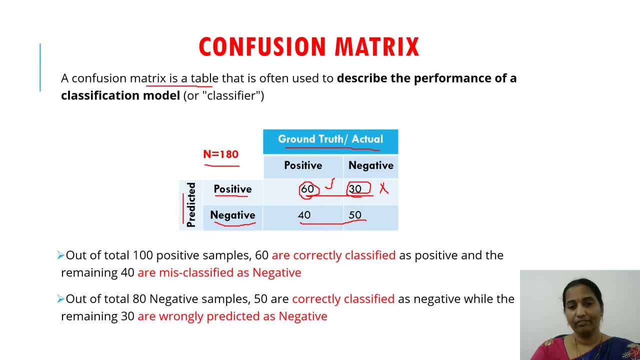 are correctly classified. and if we observe this cell, again observe this cell, So again. So these are the actually belonging to the positive class, because this column indicates the positive class in the ground truth side. that is why these 40 examples are actually belonging to the positive class, but they are predicted as negative. 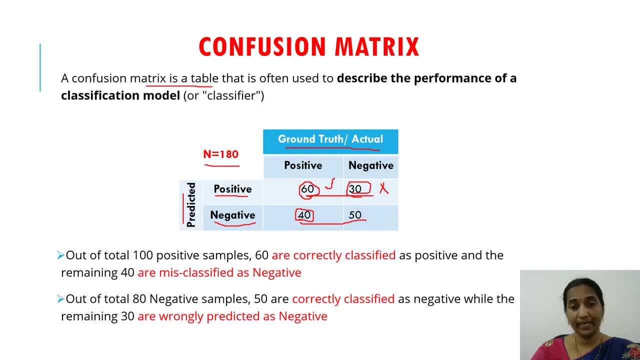 So that means positive, they are belonging to the positive class. but predicted as negative means they are again misclassified, they are wrongly classified by the model. Then look at this: these 50, the value 50. So these 50 examples, These 50 examples are actually belonging to the negative class and they are predicted. 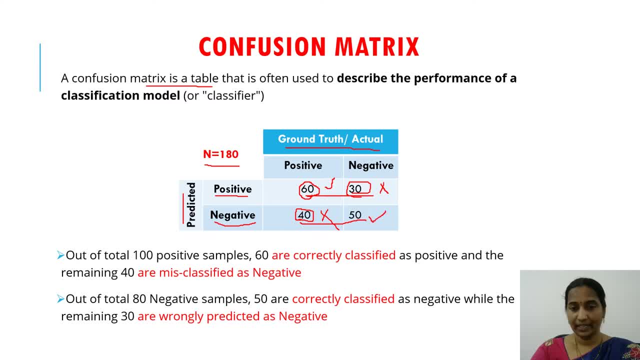 as negative also. so that means they are correctly classified. so out of the total hundred examples, how many are correctly predicted as positive? 60, and out of the 80 negative examples, how many are correct, correctly classified as negative? that is 50. and out of the hundred positive, 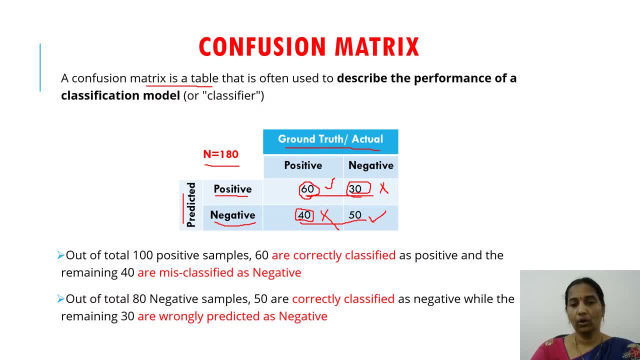 examples 40 are misclassified and similarly, out of the 80 examples, 30 are misclassified as positive by the model. So this indicates how many examples- the number of examples that are correctly classified by the model and that are misclassified by the model. 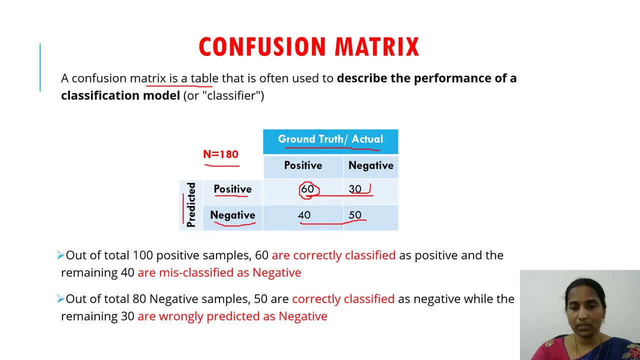 these are correctly classified. and here, if we observe this cell, the data in this cell, this indicates that actually these samples, these 30 samples, are belonging to the negative class, but they are by mistake predicted as positive by the predictor, by the model, So they are wrongly classified. that means these are wrongly classified, whereas these: 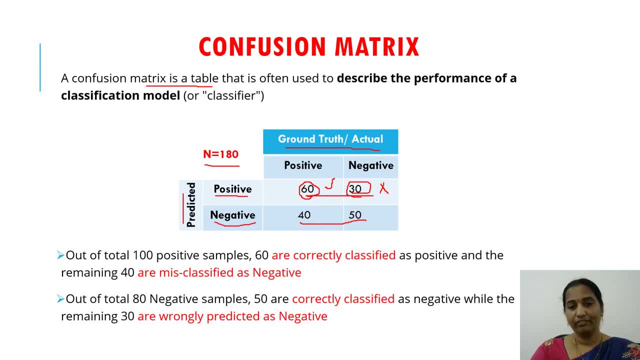 are correctly classified and if we observe this cell, again observe this cell. So these are the actually belonging to the positive class, because this column indicates the positive class in the ground truth side. that is why these 40 examples are actually belonging to the positive class, but they are predicted as negative. 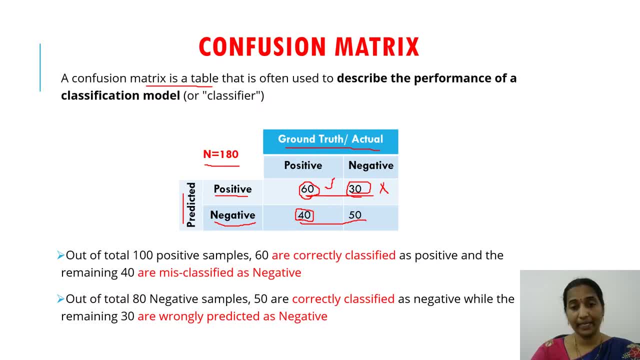 So that means positive, they are belonging to the positive class. but predicted as negative means they are again misclassified, they are wrongly classified by the model. Then look at this: these 50, the value 50. So these 50 examples, 50 examples- are actually belonging to the negative class and they are predicted as negative. 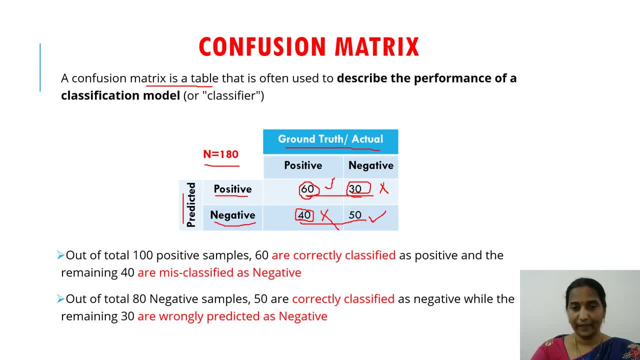 also So that means they are correctly classified. so, out of the total 100 examples, how many are correctly predicted as positive? 60, and out of the 80 negative examples, how many are correct, correctly classified as negative? that is 50. and out of the 100 positive examples, 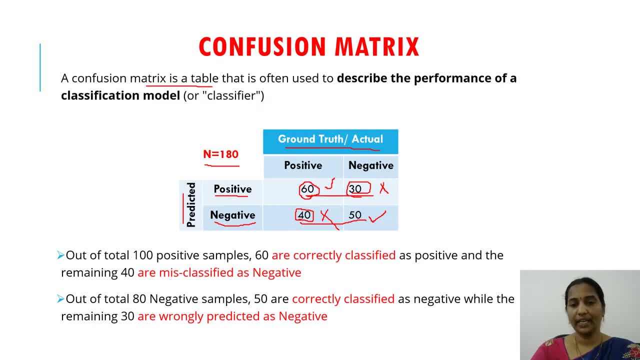 40 are misclassified and similarly, out of the 80 examples, 30 are misclassified as positive by the model. So this indicates how many examples- the number of examples that are correctly classified by the model and that are misclassified by the model. 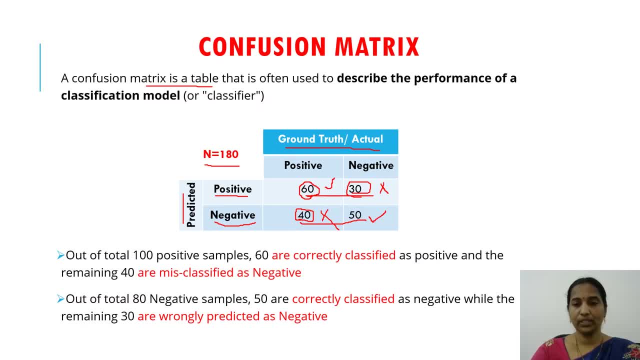 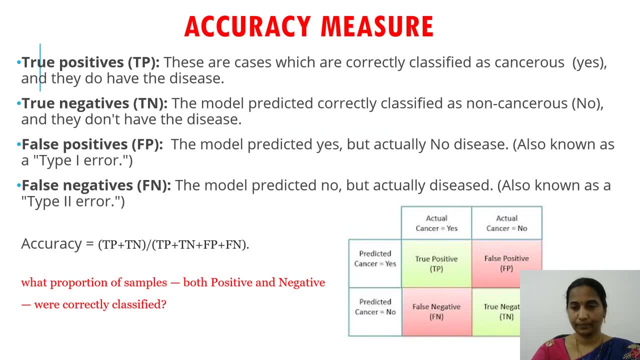 So this indicates the numbers and based on this we can measure the different matrix of the models. Let us see So here. so we are taking the cancer classification task, that is, there are two classes again. So the person is having cancer or not is the task. 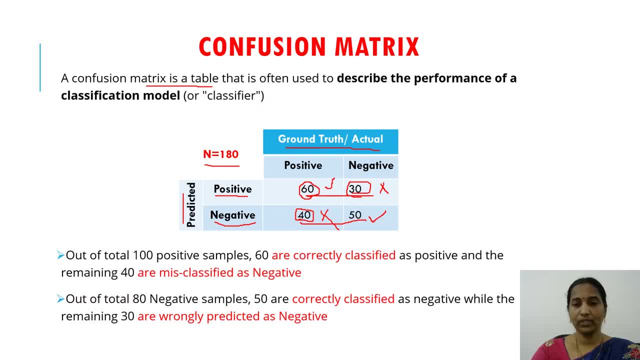 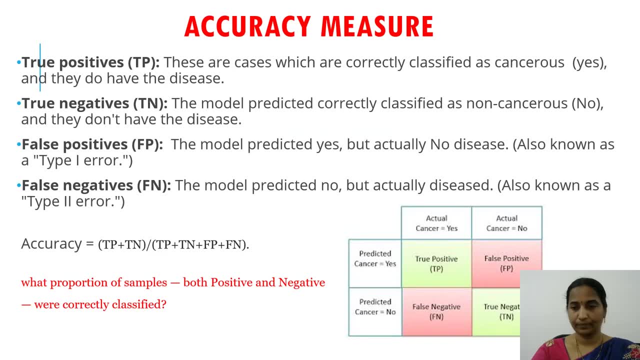 So this indicates the numbers and based on this we can measure the different matrix of the models. Let us see. So this is the number of examples, So here. so so we are taking the cancer classification task, that is, there are two classes again. 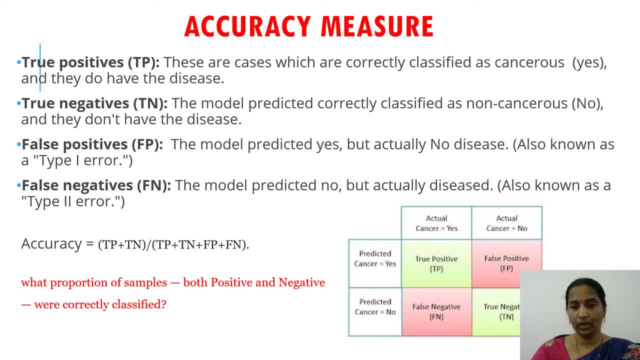 So the person is having cancer or not is a task. So in this case actual means cancer is positive, So negative means negative class indicates the cancer is. so not there in the not positive. So let us see the next example. 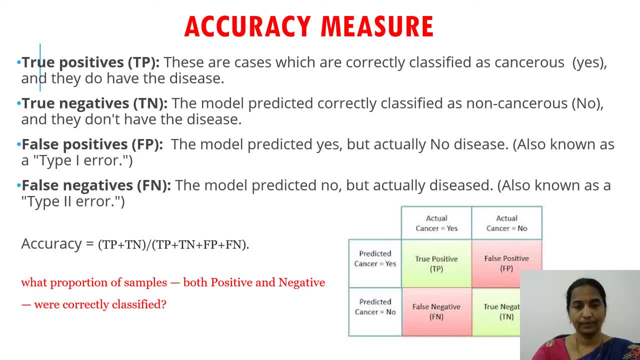 So let us see the next example. it's non-cancerous and, similarly in predicted, also cancerous, non-cancerous. there are two classes: prediction in actual and prediction. so then, so the examples that are correctly classified: they are belonging to the cancerous and they are predicted as cancerous means they are correctly. 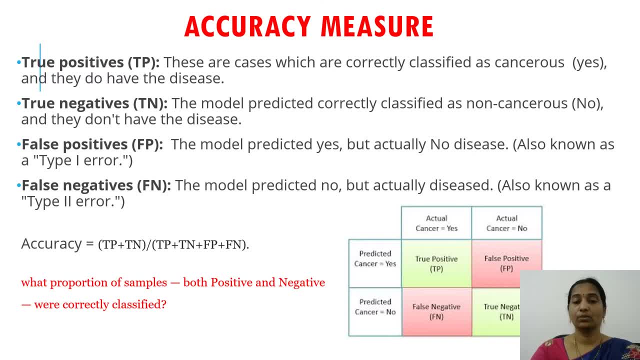 classified because they are belonging to the positive and correctly classified, we call it as true positive. the number of examples that are correctly classified as positive, we call them as true positives. and similarly, if we observe the number of examples that are belonging to the negative class and they are predicted as negative itself, that means these are also correctly. 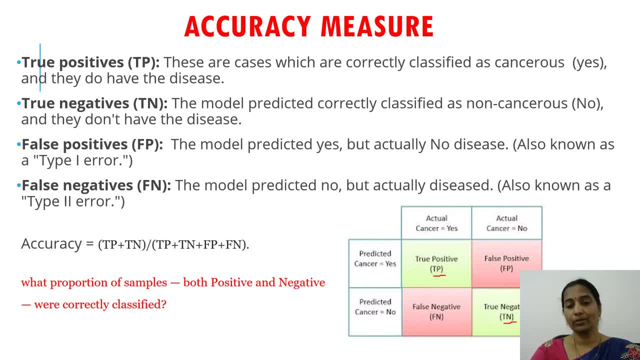 classified and we call them as true negatives. they are truly classified as negative. so that is what Tn, we shortly call it as Tn, whereas correctly classified as positive, we call it as positive, true positives. and there are other values also, those are misclassified values. So let's give 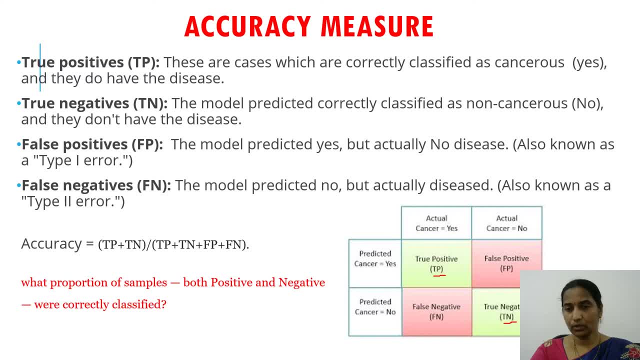 some name to that also. So this indicates, this cell indicates. so these are the actually non-cancerous cases, but they are predicted as cancers. In that case, we call them as false positive. The reason is they are falsely predicted by the model as positive. That's why we call them. 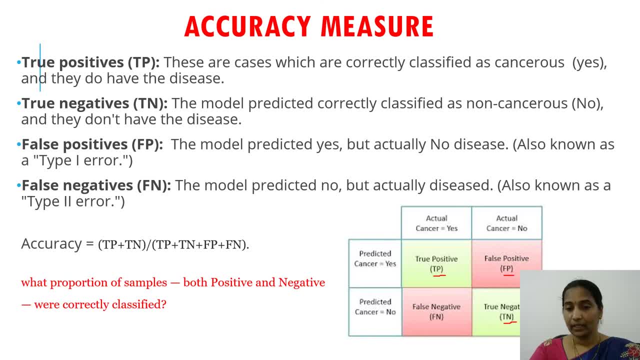 as false positives. Similarly, if we observe this number, so we call it as false negative. Again, the reason is they are actually belonging to the positive class, that is cancerous, but the model is predicting them as non-cancerous. So, falsely, the model is predicting as negative. 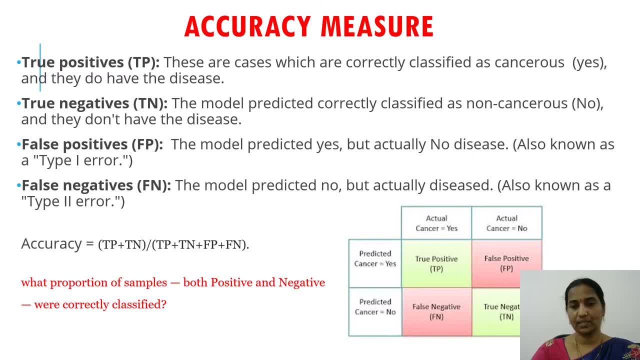 So in this case actual means cancer is positive. So negative means negative. class indicates the cancer is so not there in the not positive, It is non-cancerous, It is non-cancerous And similarly in predicted also cancerous, non-cancerous. there are two classes prediction: 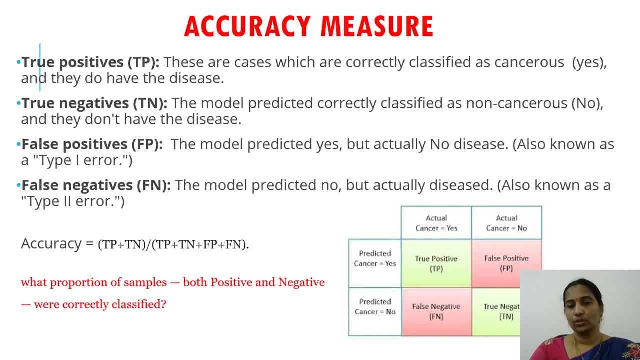 in actual and prediction. So then, so the examples that are correctly classified, they are belonging to the cancerous and they are predicted as cancerous means. they are correctly classified because they are belonging to the positive and correctly classified, we call it as true, positive. 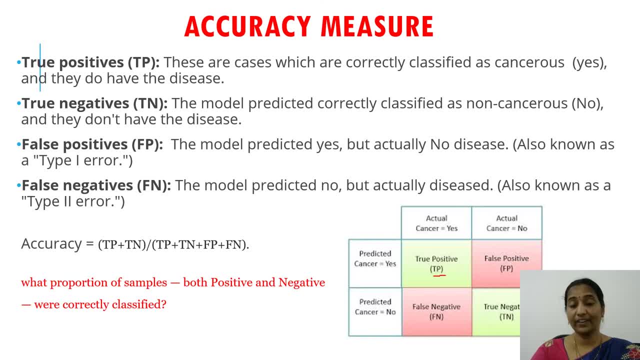 There are the number of examples that are correctly classified as positive. we call them as true positive. And similarly, if we observe the number of examples that are belonging to the negative class and they are predicted as negative itself, that means these are also correctly classified and we call them as true negatives. they are truly classified as negative. 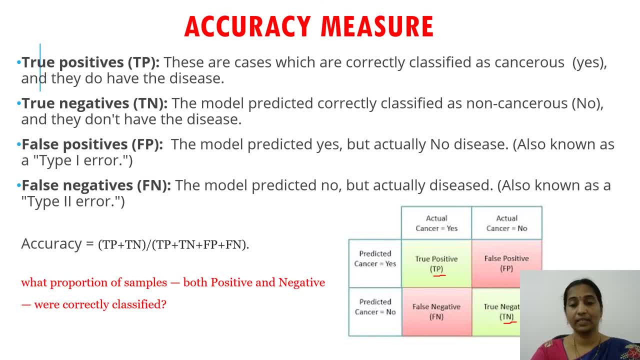 So that is what Tn, we shortly call it as Tn. whereas correctly classified as positive, we call it as true positives. and there are other values also. those are misclassified values. I will give some name to that also. So this: this indicates, this cell indicates, so this is: these are the actually non-cancerous. 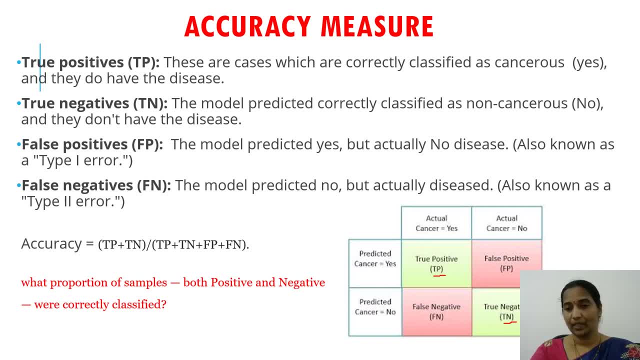 cases, but they are predicted as cancerous. In that case, we call them as false positive. the reason is: they are falsely predicted by the model as positive. that is why we call them as false positives. Similarly, if we observe this number, so we call it as false negative. again, the reason: 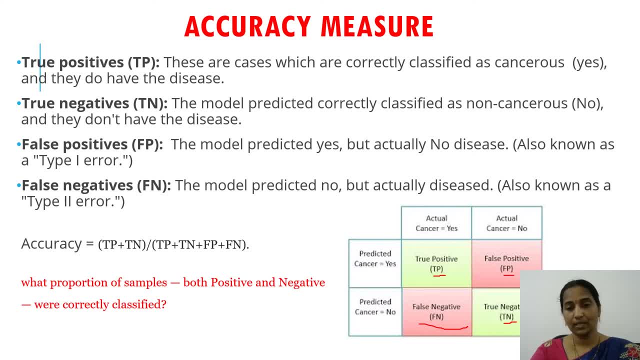 is they are actually belonging to the positive class, that is cancerous, but the model is predicting them as non-cancerous, So, falsely, the model is predicting as negative. that's why we call it as false, negative. So once we have all these values, so we can get a measure called as accuracy, which indicates 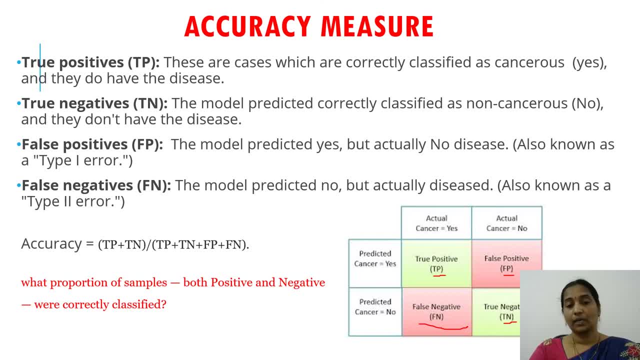 how many or what portion of the samples are actually correctly classified. So how do we get that number? so, actually, these are the numbers, these are the values that are correctly classified and these are also correctly classified. So the sum of true positives plus true negatives divided by the total number of examples, how? 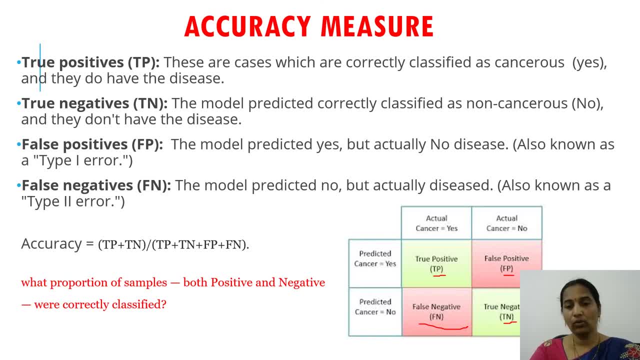 That's why we call it as false, negative. So once we have all these values, so we can get a measure called as accuracy, which indicates how many or what portion of the samples are not negative. So we can get a measure called as accuracy, which indicates how many or what. 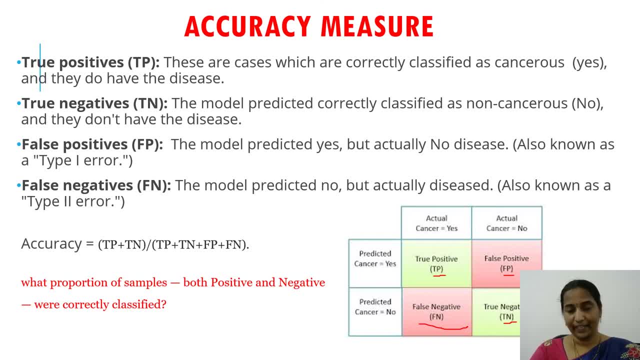 are actually correctly classified. So how do we get that number? So, actually, these are the numbers, these are the values that are correctly classified and these are also correctly classified. So the sum of true positives plus true negatives divided by the total number of examples, How do? 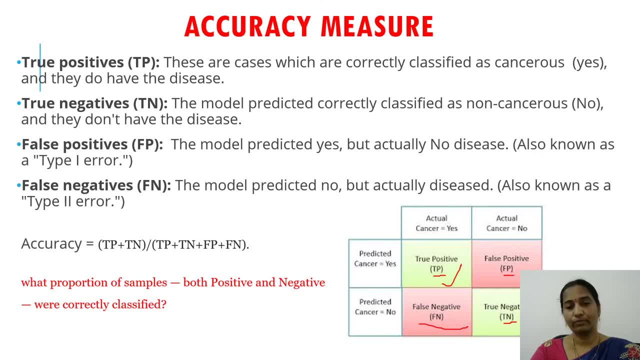 we get the total number of examples: True positive plus false positive, plus false negative, plus true negative, So sum of all these four cell values. So this is how we get the accuracy measure of a model. So what it indicates, Accuracy actually gives the proportion of the 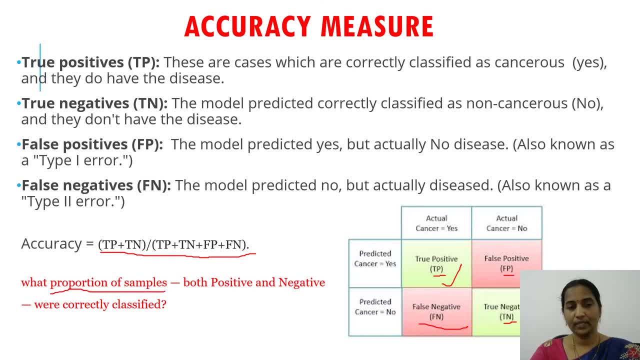 samples that are correctly classified. So usually it varies. the measure takes the values from 0 to 100. So we include the values that are belonging to both the classes, positive and negative. So in this case we are considering only binary case. The same can be. 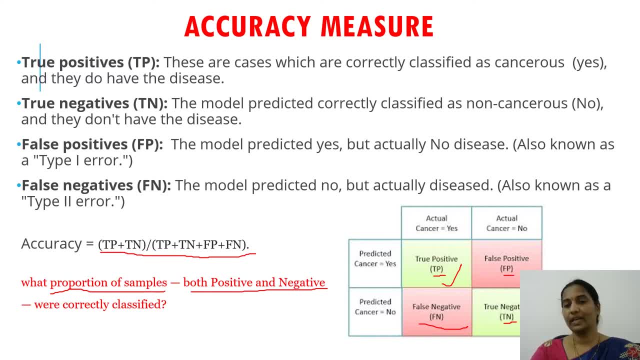 accounted for in the case of a model, So we include the values that are belonging to multiple cases also, If we have one more class- in that case we have- we will get one more row and one more column in the confusion matrix and we get the correctly classified values here and 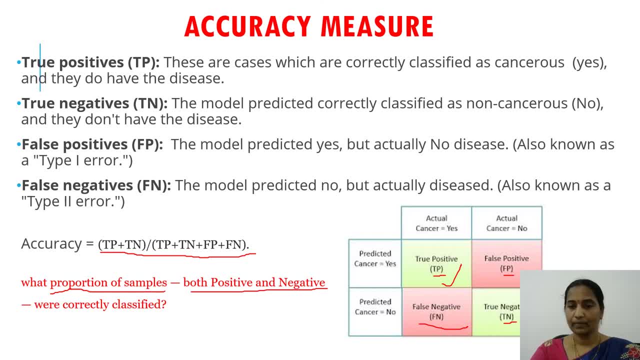 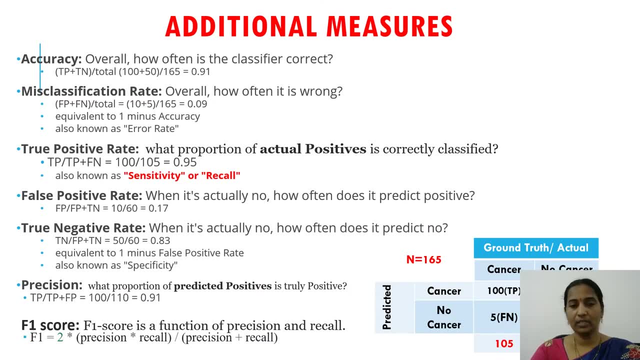 then we can get the accuracy of the multi-class classifier also And in addition to the accuracy measure. so we have various other measures also. I will shortly explain why. do we need to have all the additional metrics? Do we really need to have these additional? 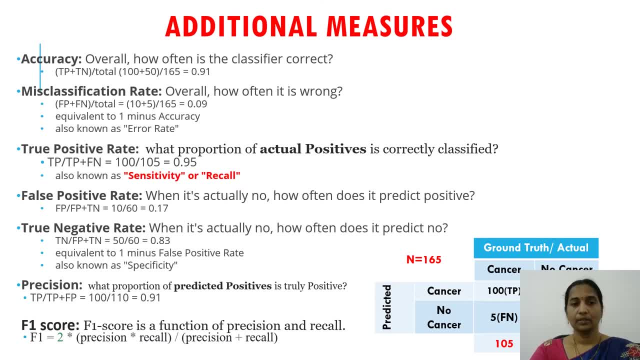 metrics or not. So I will justify that soon. So before proceeding further, let us see what are the other measures we can derive based on the confusion matrix itself. Once we have the confusion matrix, we are done with the most of the part. So once we fill the confusion matrix and 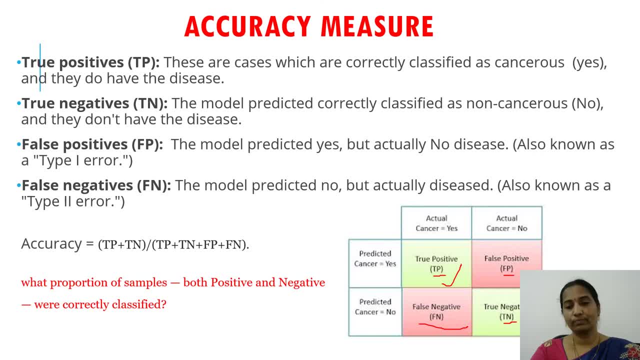 do we get the total number of examples: true positive plus false positive, plus false negative plus true negative, So sum of all these four cell values. so this is how we get the accuracy measure of a model. So what it indicates accuracy actually gives the proportion of the samples that are correctly. 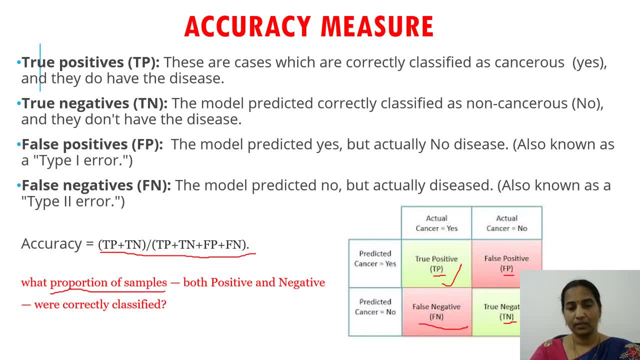 classified, So usually it varies. the measure takes the values from 0 to 100. So we include the values that are belonging to both the classes, positive and negative. So in this case we are considering only binary case. the same can be extended to multiple. 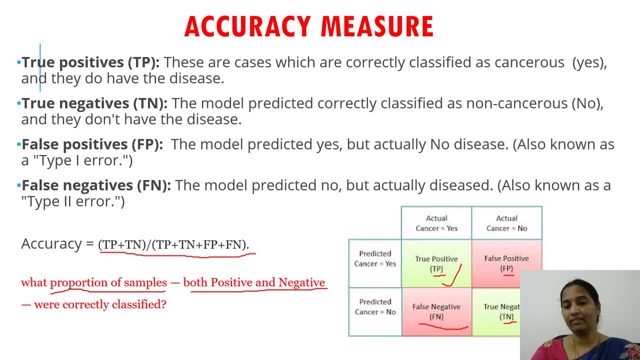 cases. also, If we have one more class- that case we have- we will get one more row and one more column in the confusion matrix and we get the correctly classified values here. So we have one more row and one more column in the confusion matrix and we get the correctly. 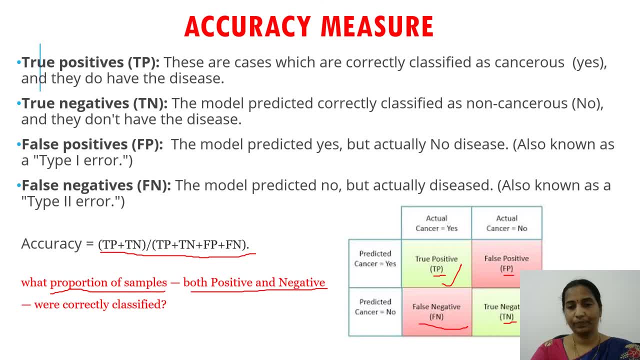 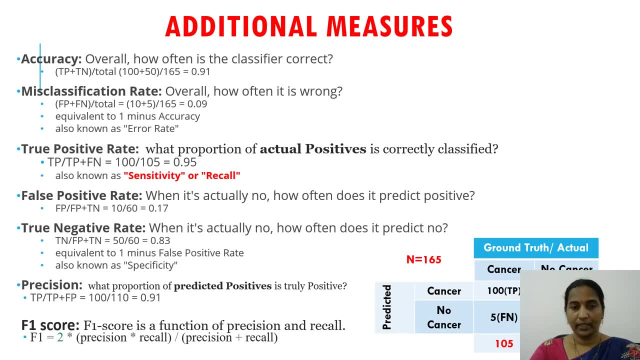 classified values here, And then we can get the accuracy of the multi-class classifier also And in addition to the accuracy measure. so we have various other measures also. I will shortly explain why. do we need to have all the additional matrix? do we really need? 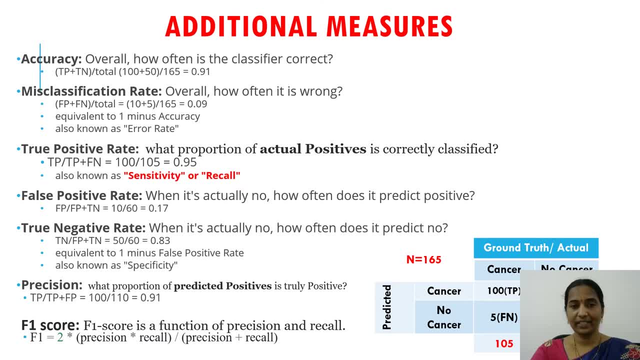 to have these additional matrix or not. So I will justify that soon. So before proceeding further, let us see what are the other measures. OK, we can derive based on the confusion matrix itself. Once we have the confusion matrix we are done with the most of the part. So once we fill the confusion matrix- and it is very easy- 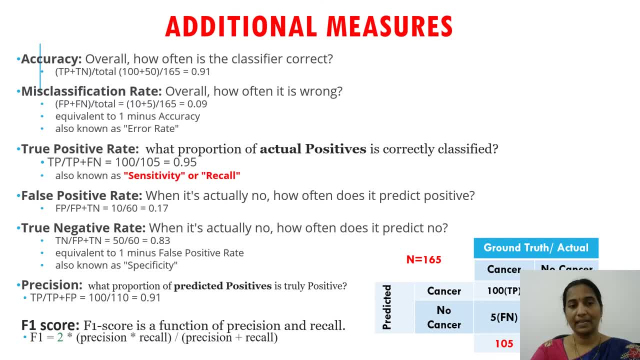 to calculate the number of measures: See here misclassification rate is the other measure. So in this confusion matrix, again we are taking the binary case and the number of examples as 165 total number of examples and 100 examples are predicted as positive, correctly classified. 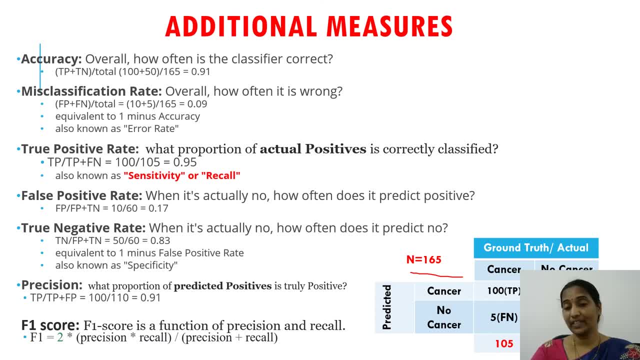 from the positive side and 50 examples are correctly classified in the negative class and similarly, the 10 examples are false positives, 5 samples are falsely predicted as negative. So once we have these values, so we can find all these measures, Let us see So: misclassification. 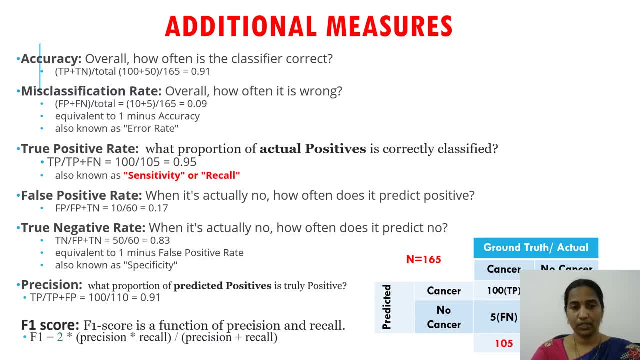 it is very easy to calculate the number of measures. See here misclassification rate is the other measure. So in this confusion matrix, again we are taking the binary case and the number of examples, as 165 total number of examples and 100 examples are predicted as positive, correctly classified. 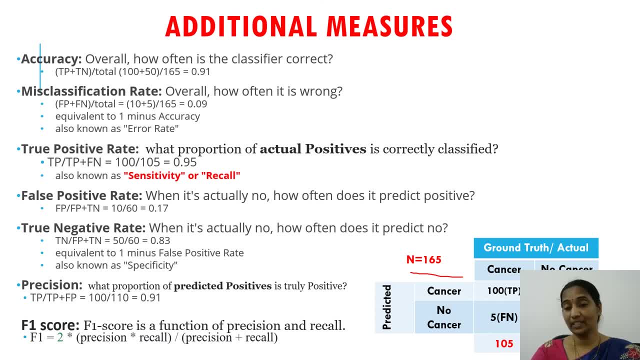 from the positive side and 50 examples are correctly classified in the negative class And similarly, the 10 examples are false positives. 5 samples are falsely predicted as negative. So once we have these values, so we can find all these measures. 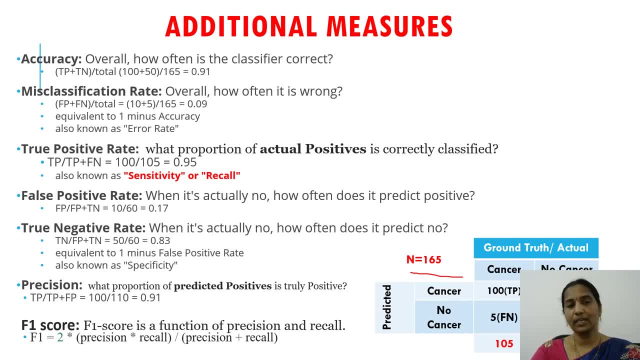 Let us see So misclassification rate. So accuracy indicates how many portion of the examples are correctly classified. In this case, 91% of the examples are correctly classified. And what is the misclassification rate? It is actually 100 minus this value, or 1 minus 0.91. 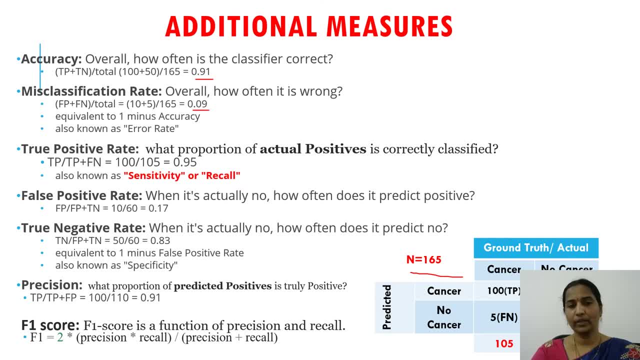 In that case it is 0.09, or you can indicate if you want it as a percentage. you can say 9%. So what this misclassification rate indicates is what are the many examples, or what portion of the examples, are wrongly predicted by the? 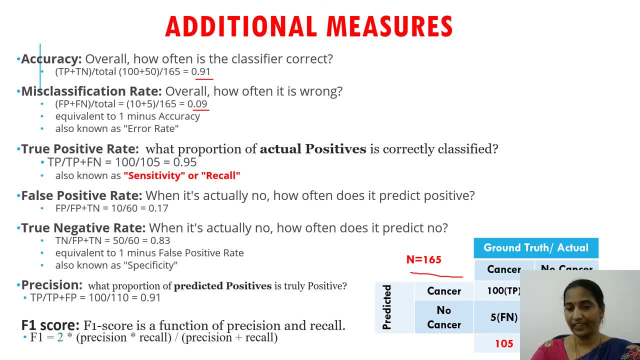 model or misclassified by the model. So what are the samples that are misclassified? the false positives and the false negatives. So it is equal to false positives plus false negatives by the total number of examples. So that gives the misclassification rate. 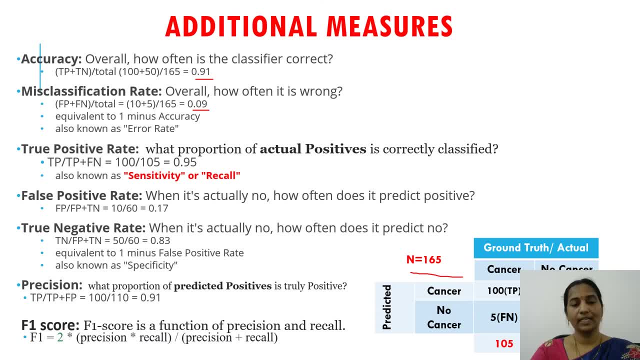 And there are other measures also. we can find all the other measures also. The next one is a true positive rate. So true positive rate. it is popularly known as sensitivity recall. actually, it tells you how many of the positive samples are correctly classified. 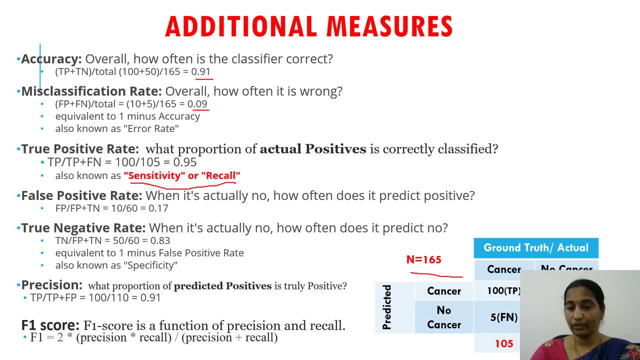 So in the ground truth, how many are belonging to the positive class? 105 are belonging to the positive class And out of those 110,, 105,, how many are correctly classified as positive? 100 are correctly classified. So in these examples, in these kind of applications, like prediction of 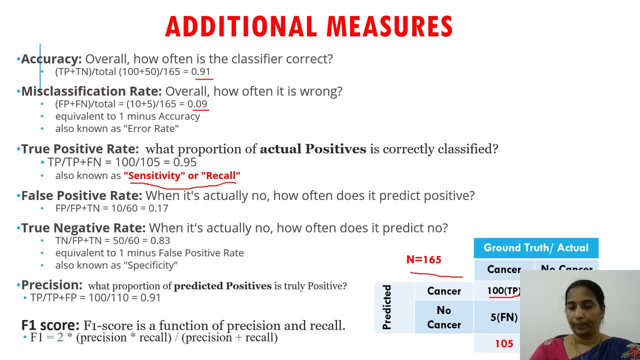 the cancer. in such applications it is very important to understand how the model is performing on the positive cases. So we are much interested in the positive cases because that is very important to understand. We should not ignore any of the positive cases. That is why. 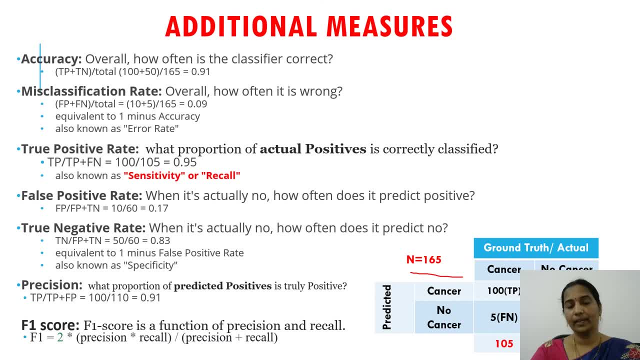 rate. So accuracy indicates how many portion of the examples are correctly classified. In this case, 91 percent of the examples are correctly classified. And what is the misclassification rate? It is actually 100 minus this value, or 1 minus 0.91.. 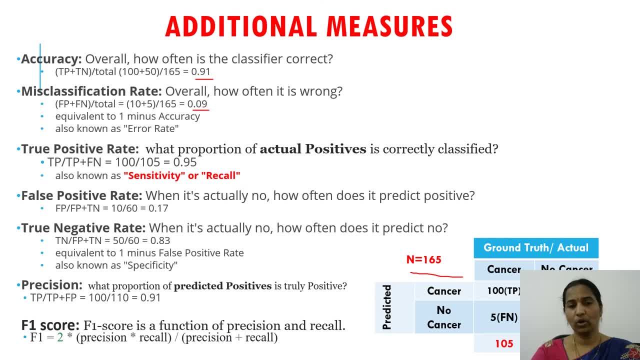 In that case it is 0.09, or you can indicate if you want it as a percentage. you can say 9 percent. So what this misclassification rate indicates is how many examples, or what portion of the examples, are wrongly predicted by the model or misclassified by the model. So what are the 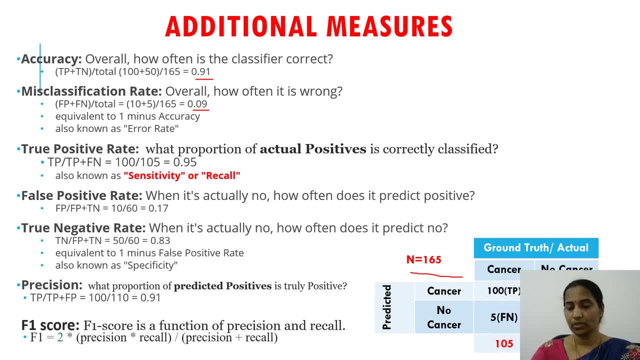 samples that are misclassified, The false positives and the false negatives. So it is equal to false positives plus false negatives by the total number of examples. So that gives the misclassification rate. And there are other measures also. We can find all the other measures. 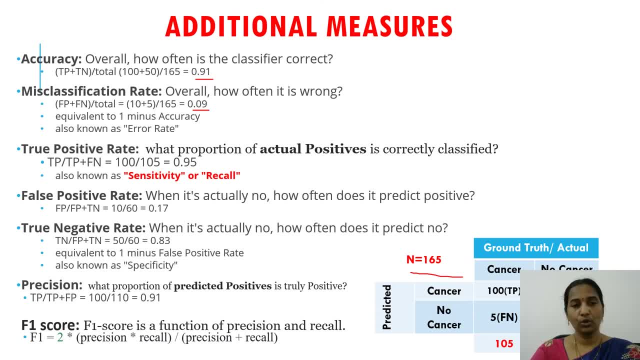 also. The next one is a true positive rate. So, true positive rate, it is popularly known as sensitivity or recall. Actually, it tells you how many of the positive samples are correctly classified. So, in the ground truth, how many are belonging to the positive class? 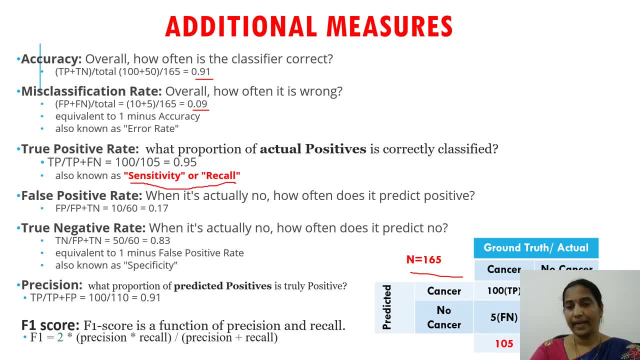 105 are belonging to the positive class And out of those 110, 105, how many are correctly classified as positive? 100 are correctly classified. So in these examples, in these kind of applications like prediction of the cancer, in such applications, it is very important. 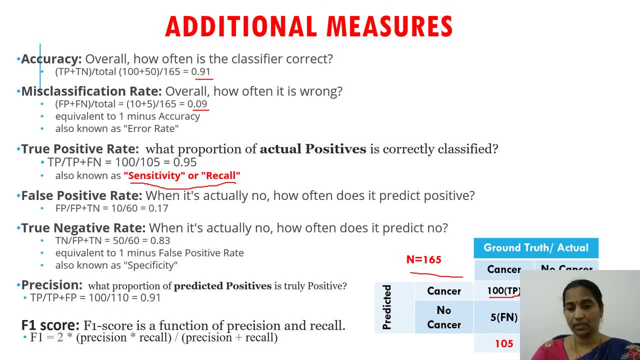 to understand how the model is performing on the positive cases. So we are much interested in the positive cases Because that is very important to understand. we should not ignore any of the positive cases. That is why we are interested in the positive cases. So recall: what it measures is how many. 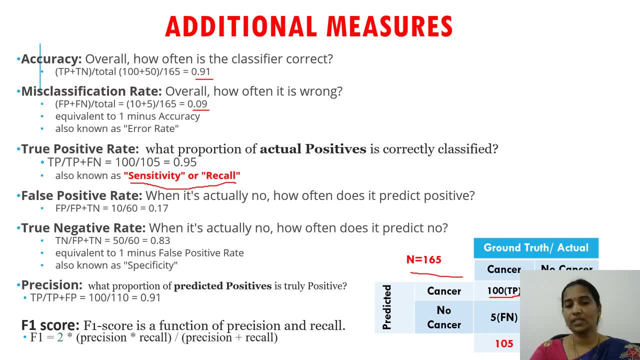 of the actual positive cases are actually predicted as positive by the model. In this case, 105 are the total samples and 100 are correctly classified as positive. So the measure is true positive by true positive plus positive, So that gives 95%. So our 95% of the positive cases are predicted by the model. So it is. 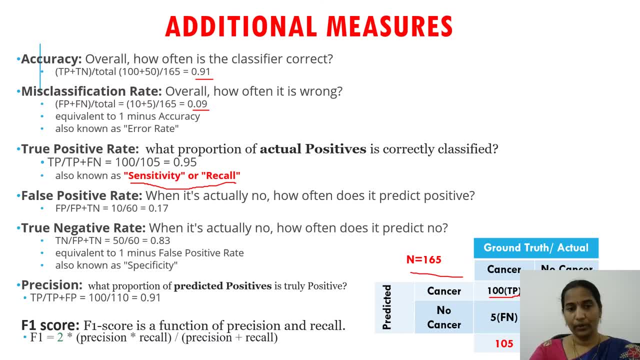 we are interested in the positive cases. So recall what it measures is how many of the actual positive cases are correct. So recall what it measures is how many of the actual positive cases are actually predicted as positive by the model. In this case, 105 are the total samples and 100 are. 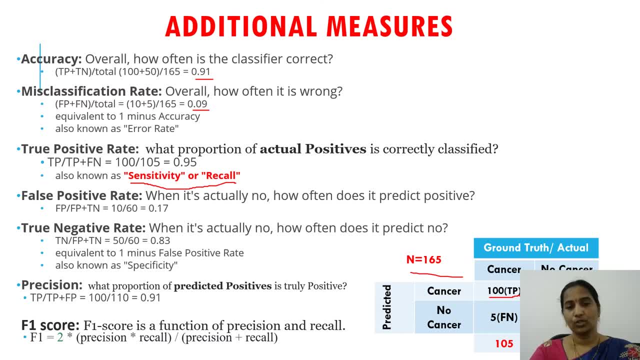 correctly classified as positive. So the measure is true positive by true positive plus false negative, So that gives 95%. So our 95% of the positive cases are predicted by the model. So it is reasonably good that means. 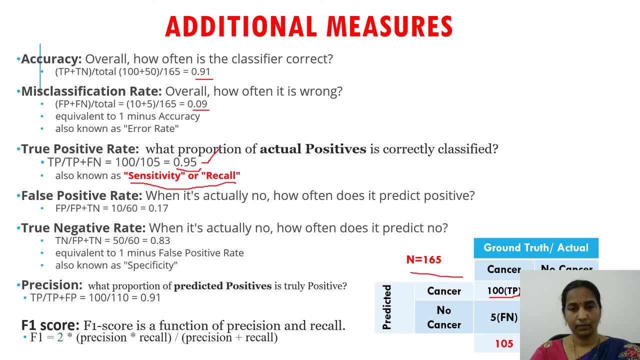 The next measure is the false positive rate. So false positive rate indicates how many of the examples are actually belonging to the samples. So false positive rate indicates how many of the examples are wrongly classified as positive out of the total negative examples. So that can be calculated as false positive rate by the total number of tantrums. 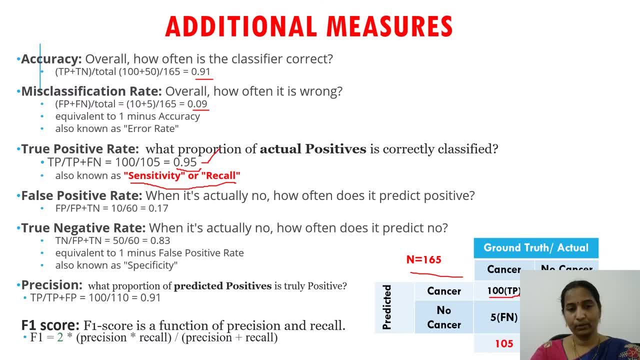 So yes, shall I calculate. So they are equal. So that is the number one: 예� MŷRЧmente. accurately, the total number of negative samples. that is a false positive rate. Similarly, we can compute the true negative rate also. True negative rate indicates. so how many are correctly classified. 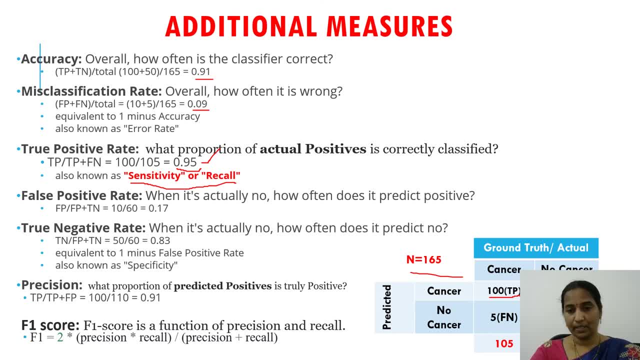 as negative out of the total negative samples. So this can be computed as true negative by the total samples that are belonging to the negative class. And another important measure is precision. So precision indicates how many of the examples are predicted as positive out of the total number of. 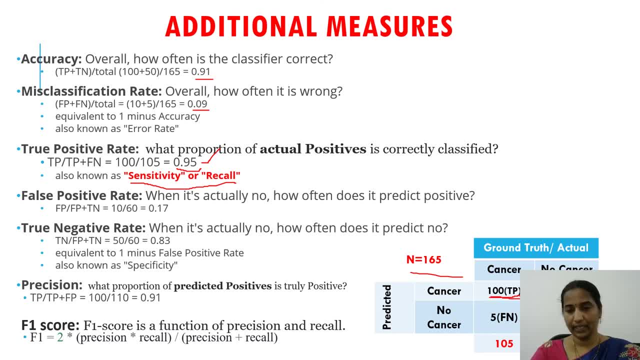 positive examples predicted by the model. that is the proportion of positively predicted examples by the model. So this is the proportion of positive examples predicted by the model. So that is what is indicated by precision. The proportion of the positively predicted examples by the model is a precision, So this can be computed as the total number of. 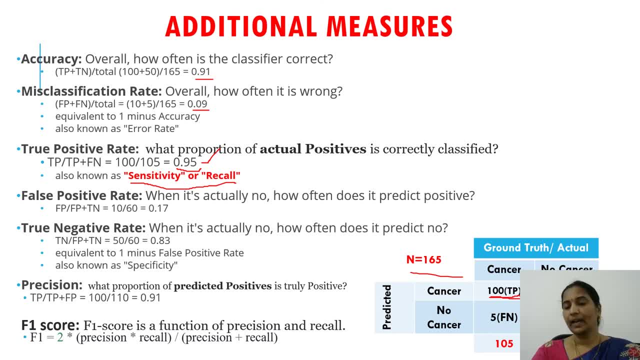 positively predicted examples are 110 and correctly classified positive examples are 100.. So 100 by 110 is equal to 91.. So 91 percent is the precision value. recall value is 95 percent. accuracy is 91 percent. 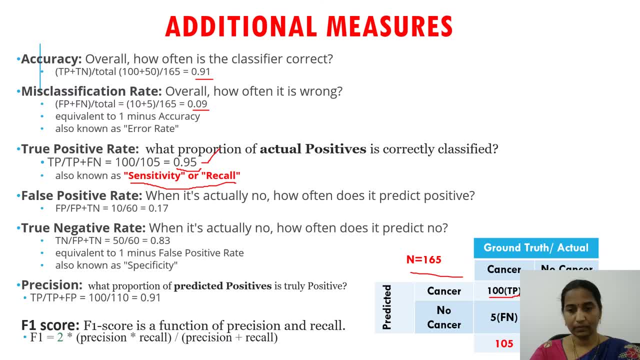 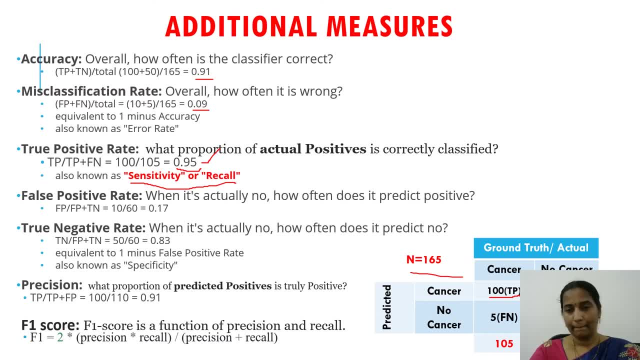 probably about n false positive people with no values. So these are according to the actual flow of data. Eye-D Vater, as we will see, is, and in mand yere. we will check this out because these are fine considered as� false positive people because 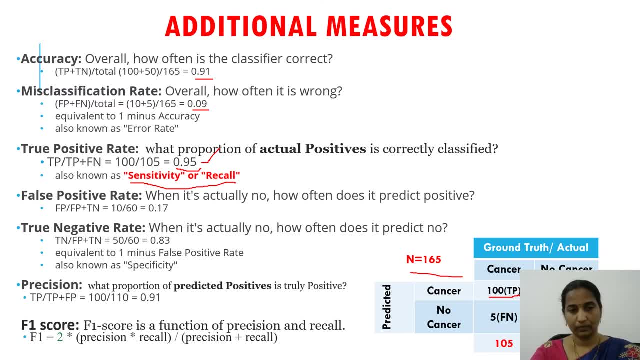 actually belonging to the false positive. a false positive rate, a false positive rate- is the predestined value of the person, So falling charge was a reason to ought tovisible control of Student- who are affected by social homes, both in common, but will monitor the. 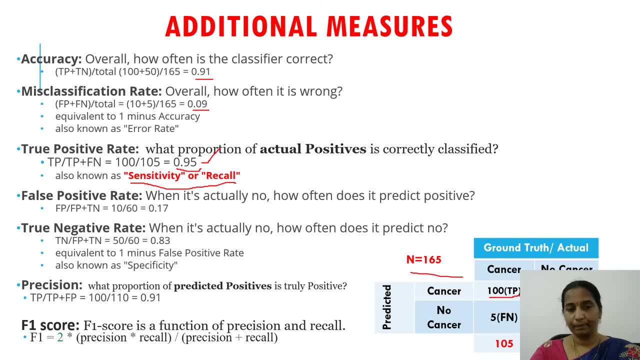 current understanding of school activities. So which will determine False positive rate? So false positive rate indicates how many of the examples are wrongly classified as positive out of the total negative examples. So that can be calculated as false positive rate by the total number of negative samples. that is a false positive rate. 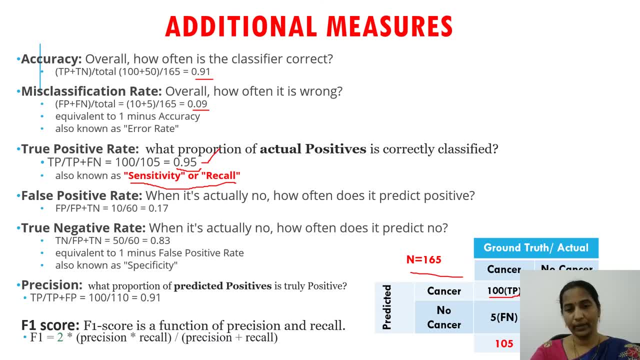 Similarly we can compute the true negative rate also. True negative rate indicates so how many are correctly classified as negative out of the total negative samples. So this can be computed as true negative by the total samples that are belonging to the negative class. And another. 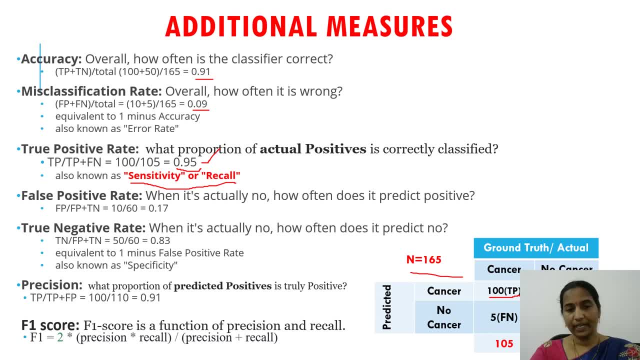 important measure is precision. So precision indicates how many of the examples are predicted as positive Out of the total number of positive examples predicted by the model. that is the proportion of positively predicted examples by the model. So that is what is indicated by precision. 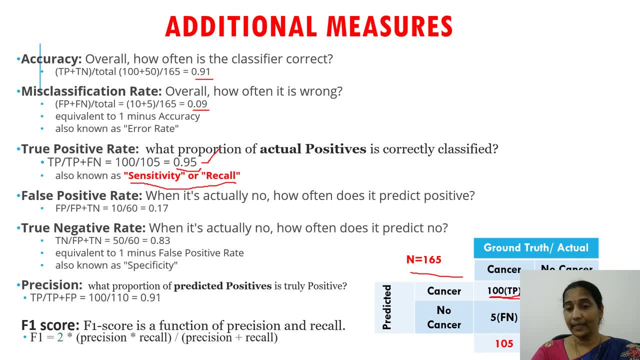 The proportion of the positively predicted examples by the model is a precision, So this can be computed as the total number of positively predicted examples are 110 and the possitive examples are 100.. You can use this with any 2002 measure менее JJ. 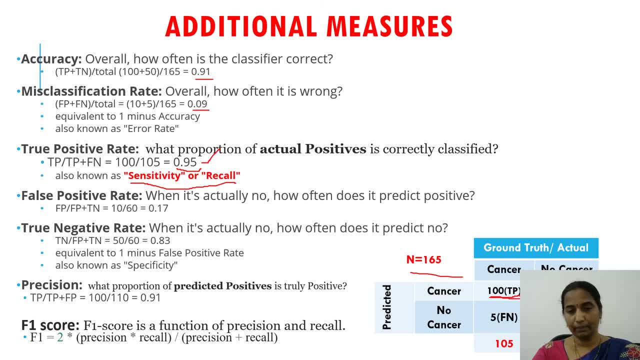 So that 100 By 110 is equal to 91. This is the quicker stage of the process. So 81% is the precision value, recall 25 res And accuracy is 91%. f1 score is another useful measurement. 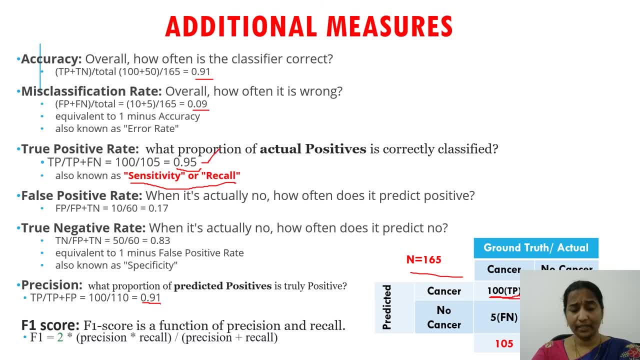 F1 score. So F1 score is another useful measure to indicate the performance of a classifier. So this is actually a combination of. this measure is actually a combination of precision and recall. So sometimes precision or recall may not give good indications, So we will shortly see when they fail Even accuracy. 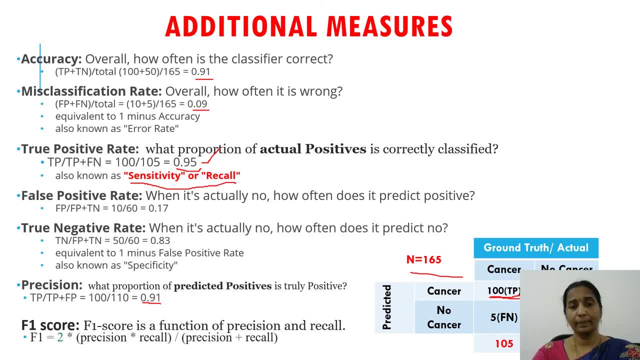 also fails in certain cases. We will shortly see when accuracy, precision, recall may not be good indications, So we will shortly see when they fail. So we will shortly see when they fail. So we will shortly see when they fail. So in that case we better go for. 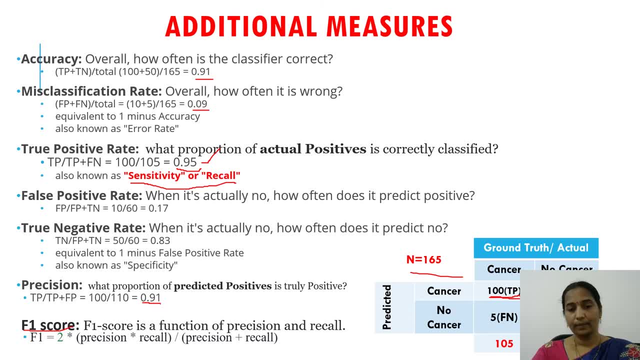 F1 score. So F1 score indicates the overall performance of the model. So this can be computed as 2 into precision, into recall. by precision plus recall, This is actually a harmonic mean of precision and recall of the model. This is how we can compute different. 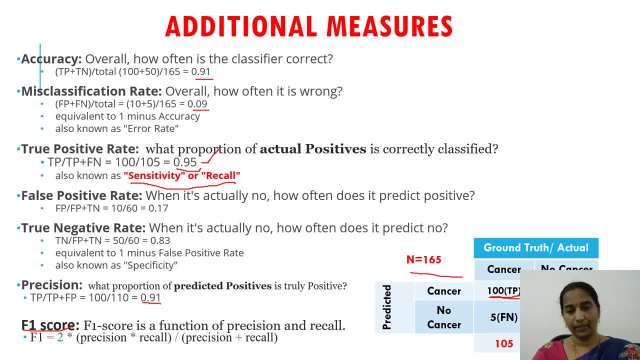 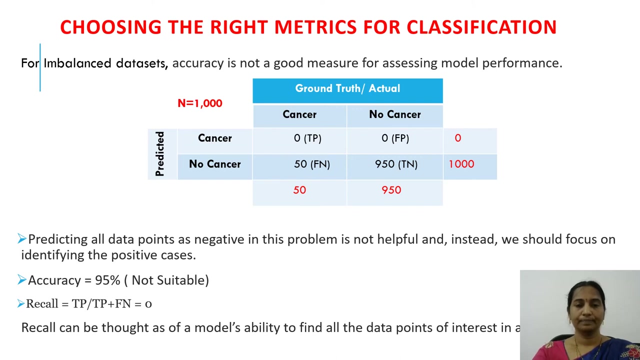 performance measures once we have the confusion. So it is very important to understand the confusion matrix, how to prepare the confusion matrix, how to fill the table and once we have the values, we can easily measure various performance measures. Now we have seen different performance measures and how to compute different. 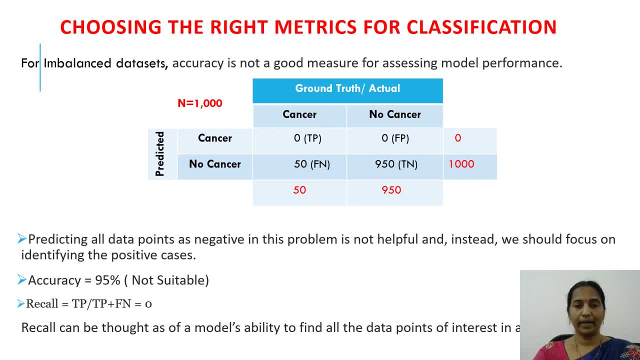 performance measures based on the confusion matrix, Then when to use which measure? So his accuracy is not sufficient to measure the performance of a classification model. Now, in certain cases, accuracy is not a good measure, especially when the data set is an 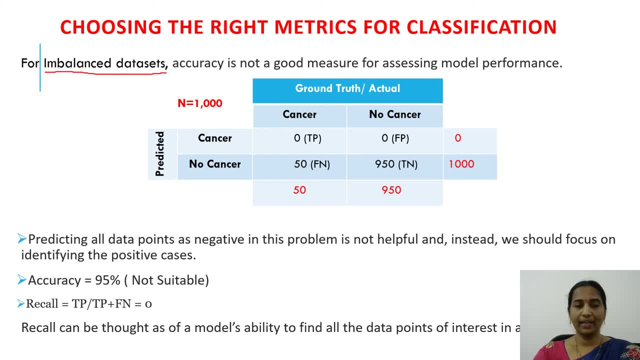 imbalanced data set. So a data set is imbalanced means the number of samples available in all the classes is not balanced. that means not equal in number. So consider this case. So there is an application for cancer classification again. So in a real-time scenario. so if we consider the 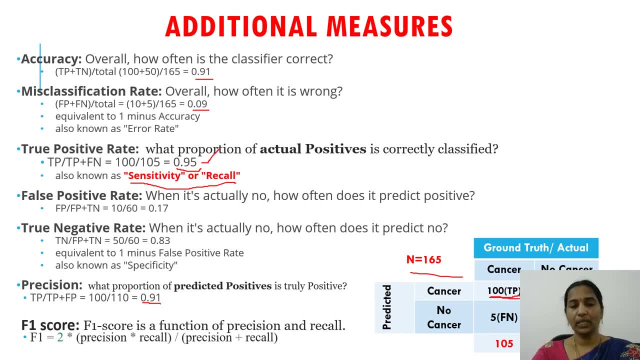 So to the performance of the classifier. So this is actually a combination of this measure. This is actually combination of precision and recall. Last ", precision or recall may not give good indications, So we will shortly see when they fail. Even. 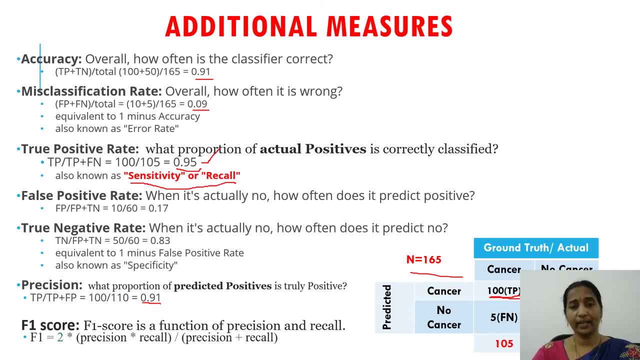 accuracy also fails in certain cases. We will shortly see when accuracy, precision, recall may not be good indicators, So in that case we better go for F1 score. So F1 score indicates the overall performance of the model. So this can be computed as 2 into precision, into recall. 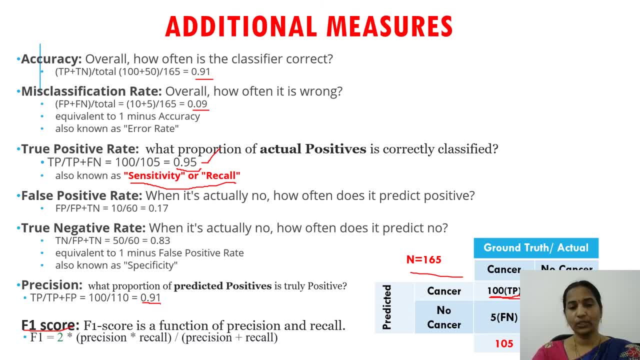 by precision plus recall. This is actually a harmonic mean of precision and recall of the model. This is how we can compute different performance measures once we have the confusion matrix. So it is very important to understand the confusion matrix, how to prepare the confusion. 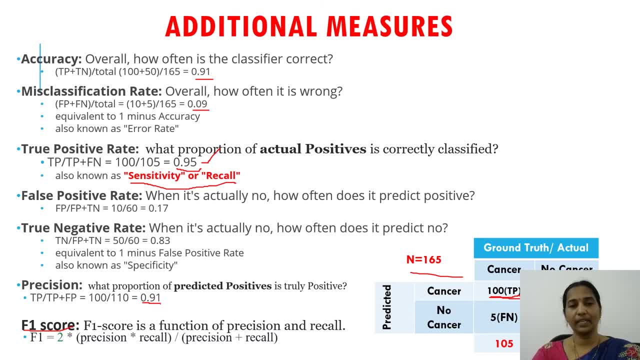 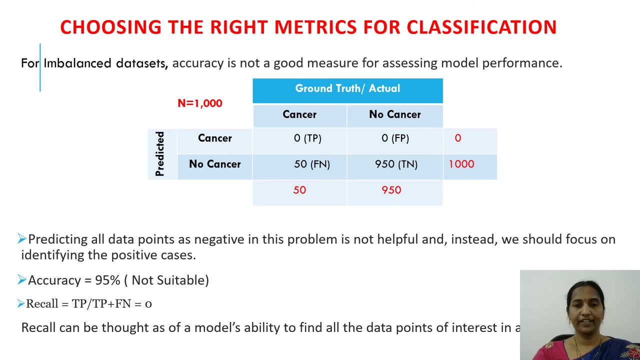 matrix, how to fill the table, and once we have the values, we can easily measure various performance measures. Now we have seen different performance measures and how to compute different performance measures based on the confusion matrix, Then when to use which measure. So is accuracy is not sufficient. 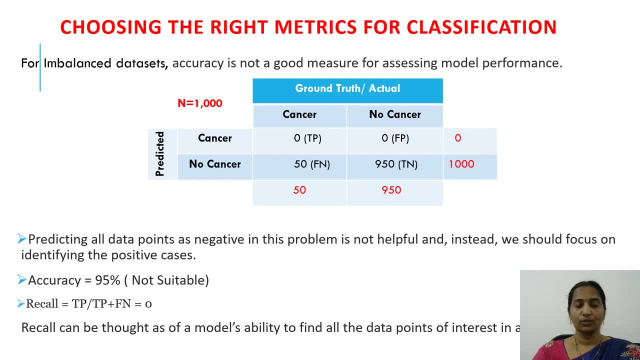 to measure the performance of a classification model. So in certain cases accuracy is not a good measure, especially when the performance is not good. So we have seen different performance measures. Now we are going to look for Equivalenteldatacet of. we have seen 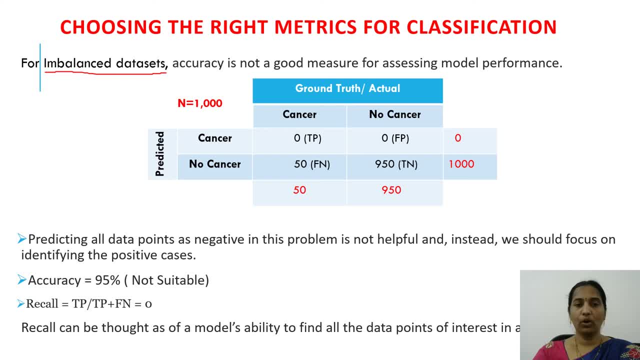 that the preparation itself is acceptable for some analysis in comparison to non- Evans gift algorithm. So we are going to look forPiercing Garlic2 Uh. Dating analysis, Cap 2. Show umasional values On yi yi yi Before we and after doing research on e to b's method. 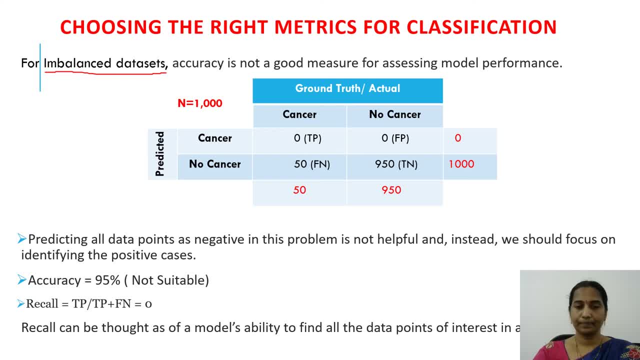 people, so rarely this disease is affected. So out of the, I have taken 1000 samples out of the 1000 samples. so 950 are negative and 50 are positive. So they are identified as cancerous and remaining are identified as non-cancerous. So if we observe the prediction, 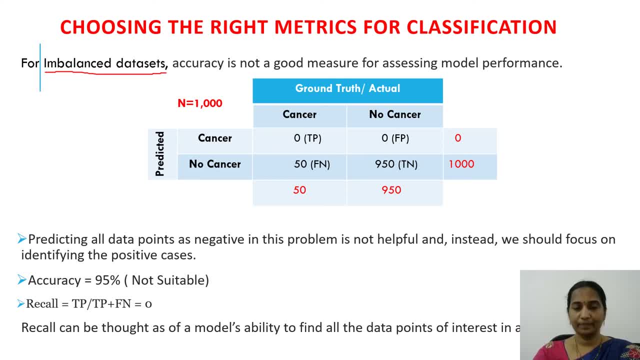 of the model so I am taking. I am not basically applying any machine learning algorithm, So I have taken a model which basically predicts every example as non-cancerous. So that is what the model I have taken. So in this case, if we observe so, 50 examples are: 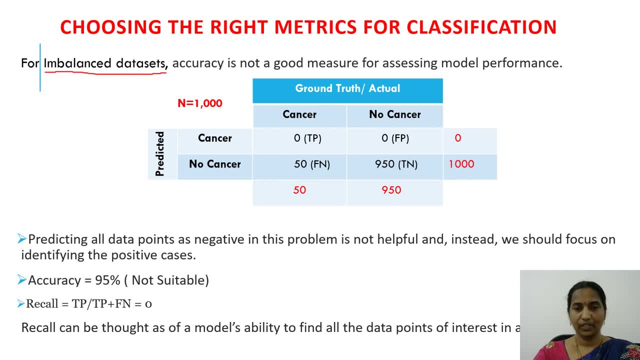 actually cancerous and 950 are non-cancerous. So I smartly what I did is I assign all the examples. I observed that most of the examples are belonging to the non-cancerous case, So even if I assign all the examples to the non-cancerous case also, so I will get 95%. 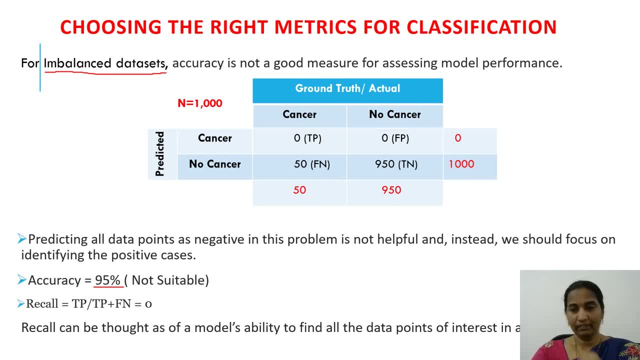 accuracy. So as I observed that to give a hype on the accuracy measure, so without putting any effort, so I created a model such that every example I get is determined as non-cancerous. So even if I do that, my accuracy measure is 95%. Is it a good indicator? now, No, right. So 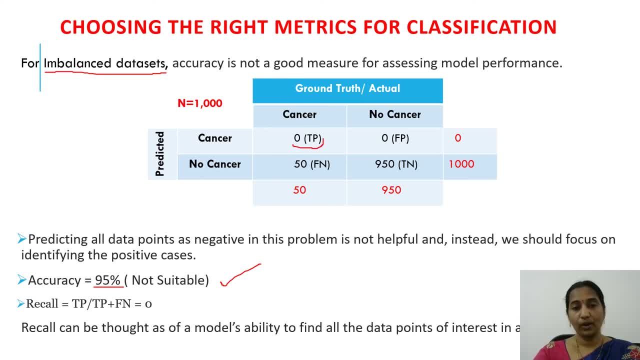 actually we are much interested in the positive cases, but the model is actually showing there are no cancerous patients at all. So now the model is failing. In these cases especially, accuracy is not a good measure. In such cases, we can rely on a metric or a measure called as recall. 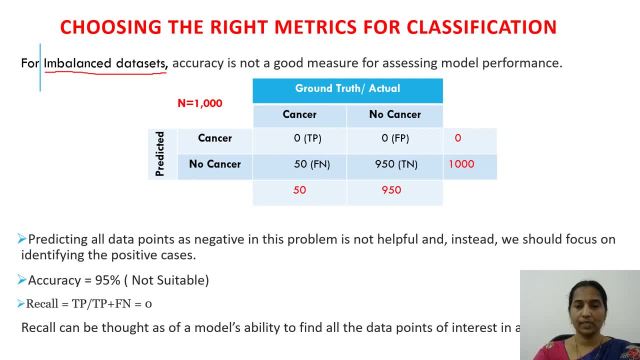 out of the. I have taken 1000 samples out of the 1000 samples. so 950 are negative and 50 are positive, So they are identified as cancerous and remaining are identified as non-cancerous. So if we observe the prediction of the model, so I am taking 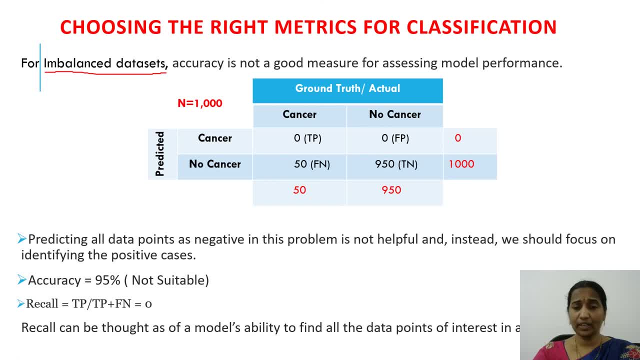 I am not basically applying any machine learning algorithm, So I have taken a model which basically predicts every example as non-cancerous. So that is what the model I have taken. So in this case, if we observe so, 50 examples are actually cancerous and 950 are. 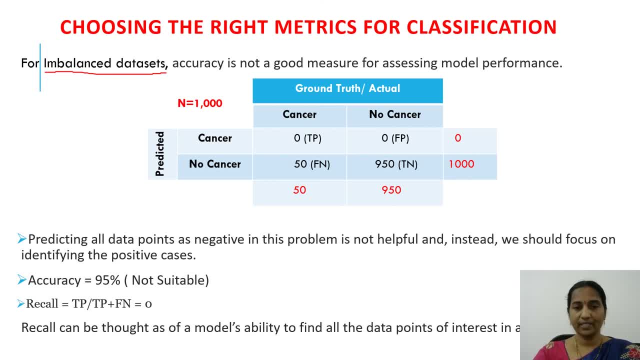 non-cancerous. So I smartly what I did is I assign all the examples. I observed that most of the examples are belonging to the non-cancerous case, So even if I assign all the examples to the non-cancerous case also, so I will get 95%. 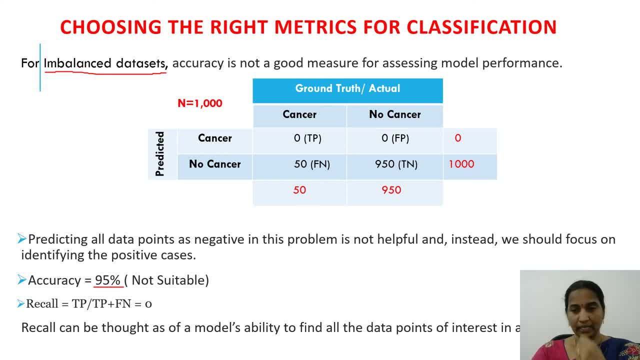 accuracy. So as I observed that to give a hype on the accuracy measure, so without putting any effort, so I created a model such that every example I get is determined as non-cancerous. So even if I do that, my accuracy measure is 95%. Is it a good indicator? now, No right. So if I do that, my accuracy measure is 95%, Is it a good indicator? now, No right. So even if I do that, my accuracy measure is 95%, Is it a good indicator? now, No right. 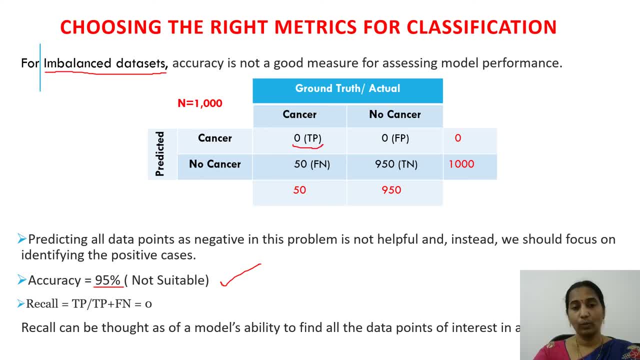 So actually we are much interested in the positive cases, but the model is actually showing there are no cancerous patients at all. So now the model is failing. In these cases especially, accuracy is not a good measure. In such cases, we can rely on a metric or a measure called as. 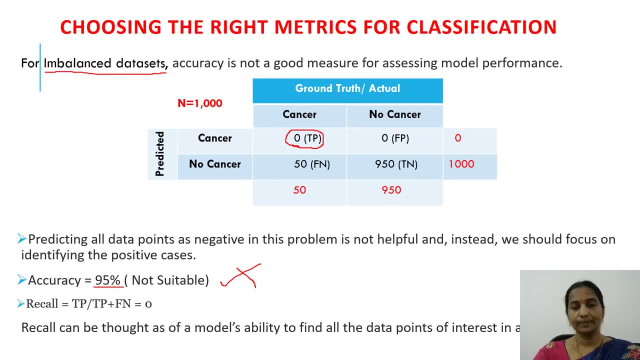 recall. So recall what it tells is a measure called a recall. So recall what it tells is a measure called a recall. So recall what it tells is a measure called a recall. So recall what it tells is. 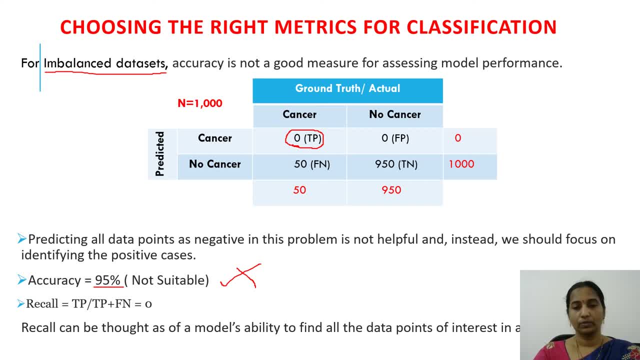 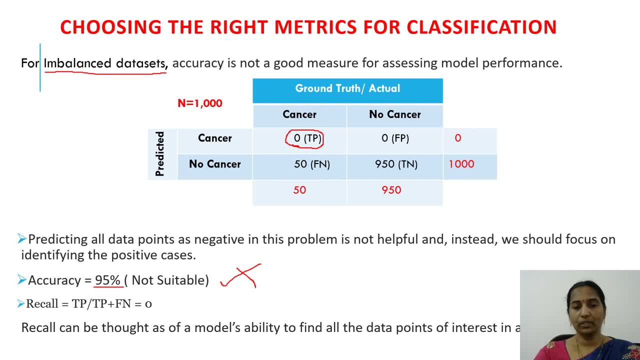 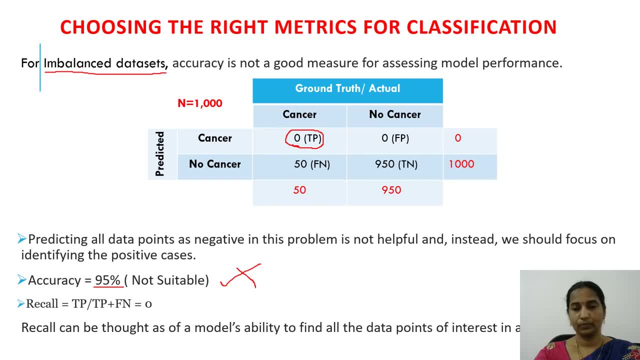 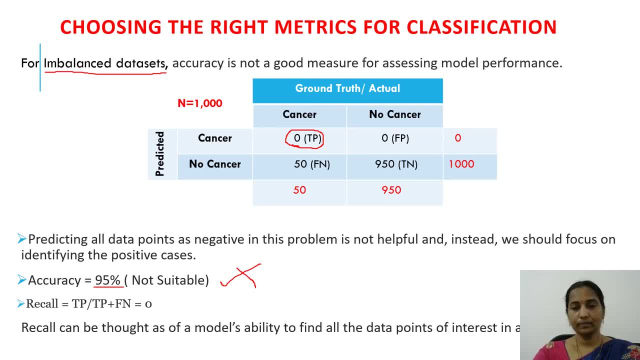 So recall what it tells is recall tells. so how many portion of recall tells us what portion of the interested points are correctly classified? In this case we are interested in true positives. So out of the positive case, how many positive points are? 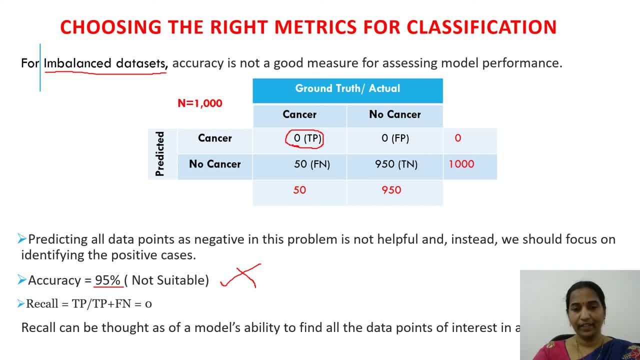 correct how many are positively classified. So if we consider that measure, so true positive by true positive plus false negative, that is 0 by 0 plus 15, that is 0 by 50 is 0.. So now, when we look, 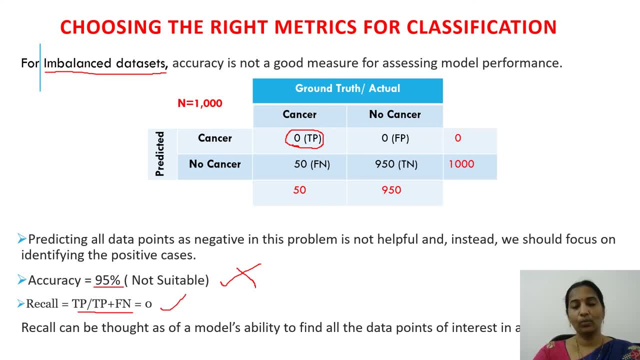 at the recall. so it clearly indicates that our model is not at all performing well, Whereas if we rely on accuracy alone, we feel that our model is performing excellent. So in these cases we better rely on recall. So the data 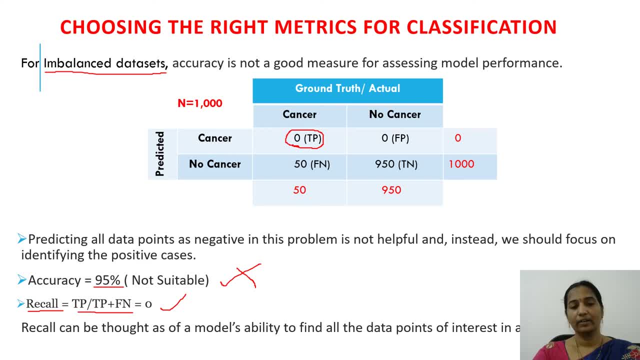 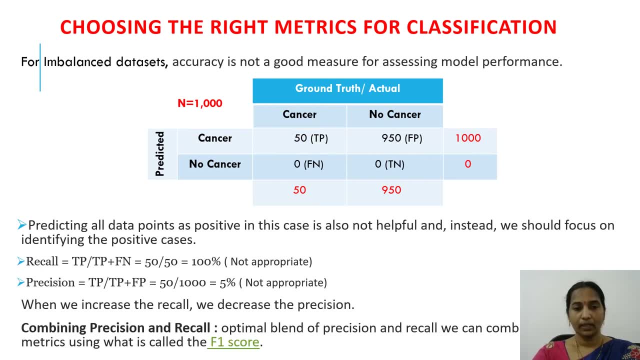 when the data sets are imbalanced, then we better rely on recall, not on accuracy alone. Now let us take another example. Now I have changed. I have taken the same example, but I have changed the model. So what I did is what I did is. so, instead of assigning every 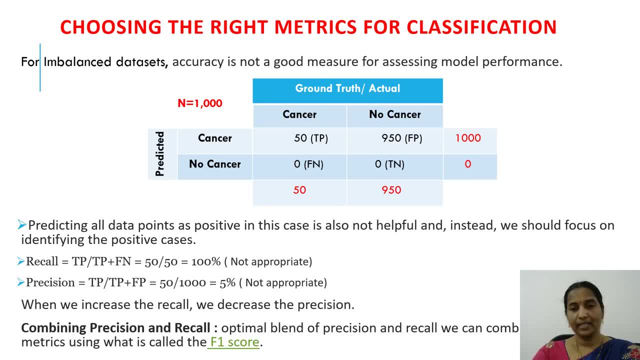 example, to the positive class. I assigned every example, every set of examples, to the positive class. So instead of finding every sample as cancerous, so as i observed that the customer is more interested in the true positive case, so i smartly assigned every example that comes to me as a positive sample. 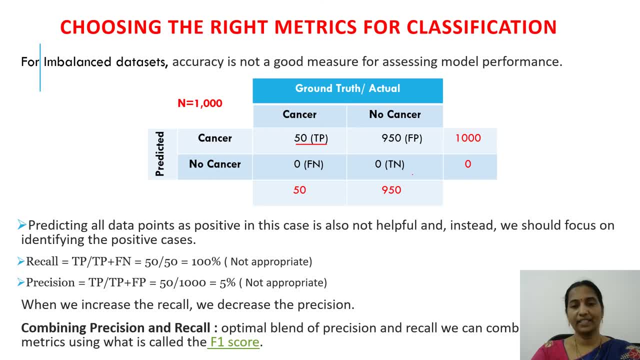 so, instead of looking into the example, i simply classify it as positive. so as so, i have taken the advantage of the customer's interest and i classified them as cancerous. so now, if we rely on the recall alone, then will it be appropriate? so if we call, if we consider the recall of the 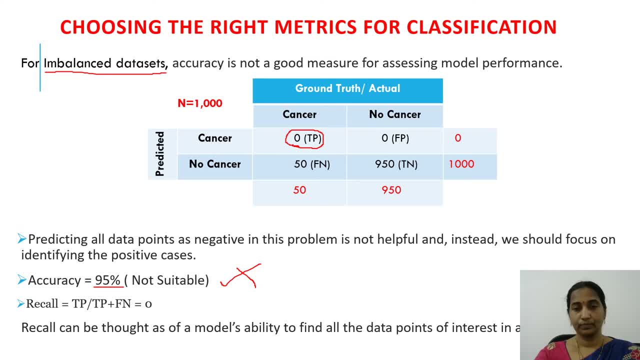 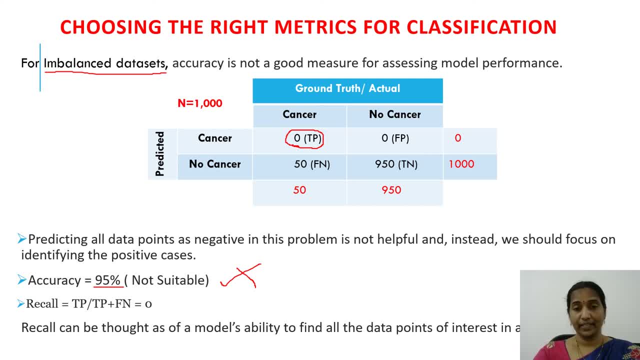 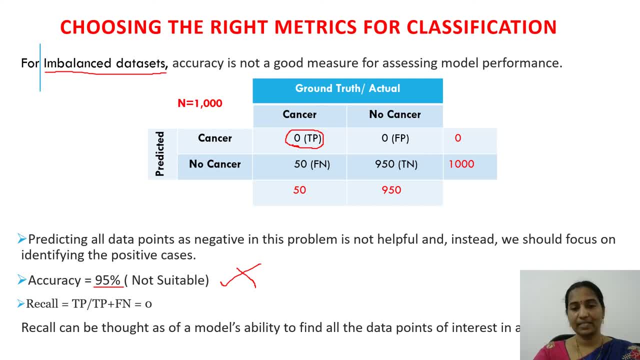 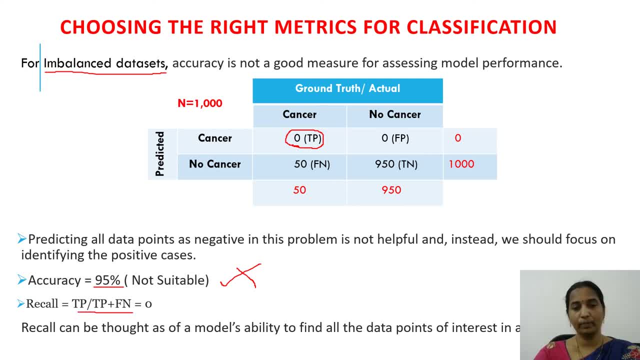 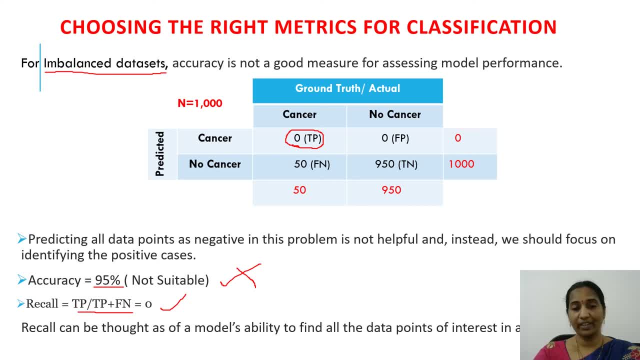 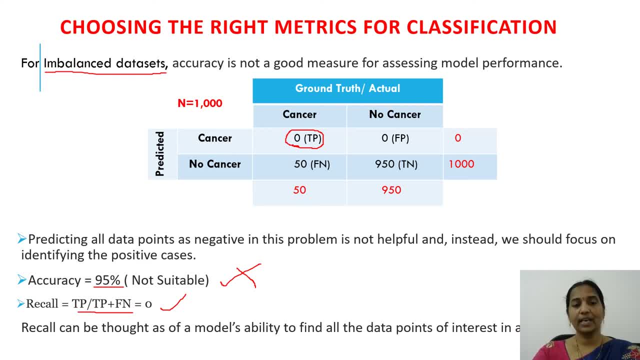 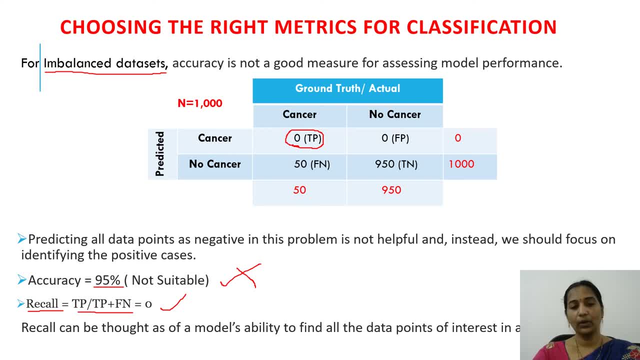 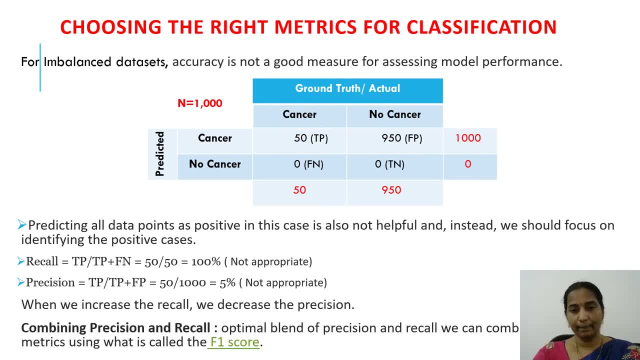 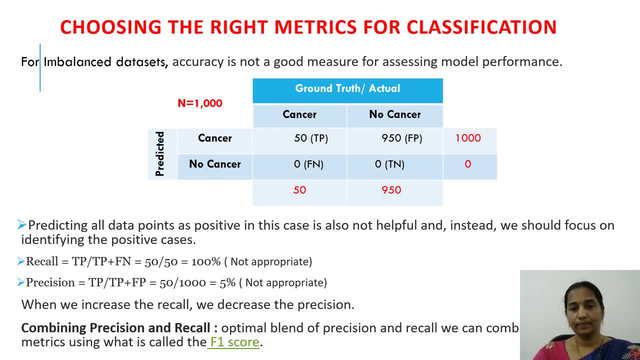 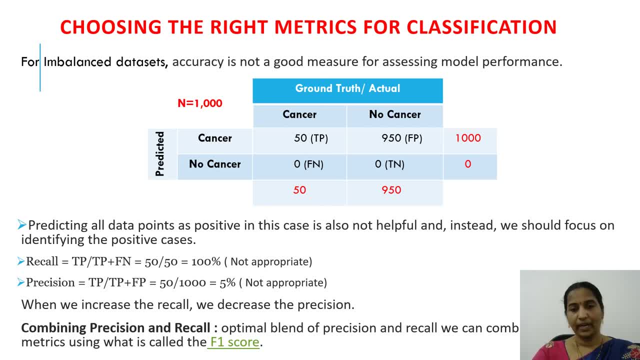 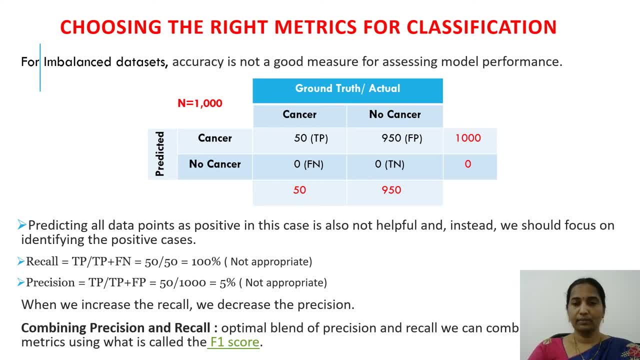 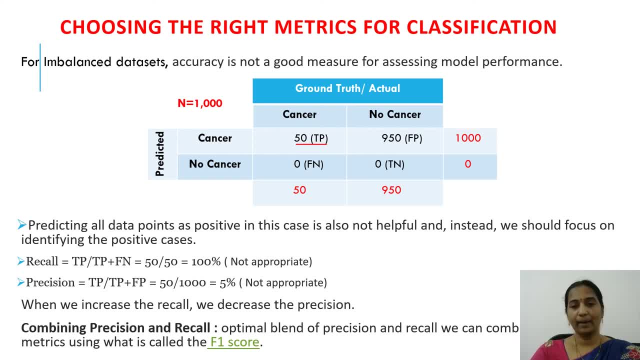 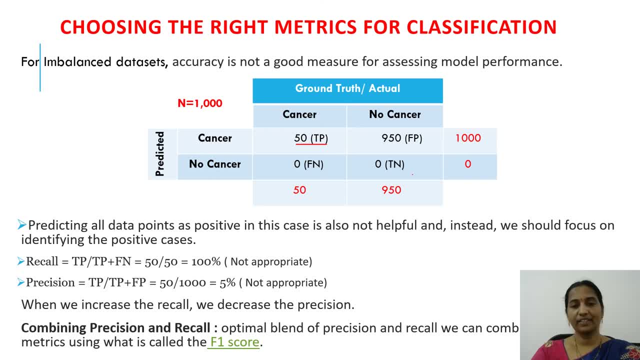 a measure called a recall. So recall what it tells is a measure called a recall. So recall what it tells is a measure called a recall. So recall what it tells is. so I have taken advantage of the customer's interest. 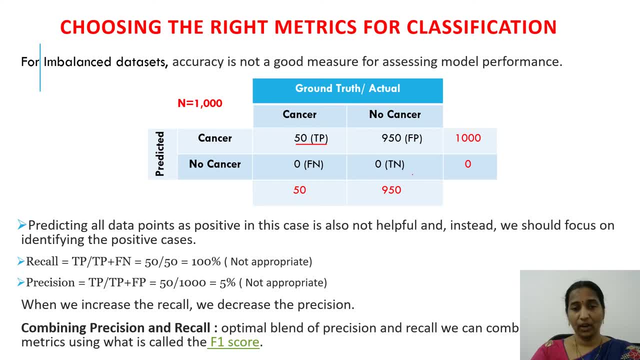 and I classified them as Cancerous, and I classified them as Cancerous. So now, if we rely on the recall alone, then will it be appropriate? So if we consider the recall of the model, it shows 100%. The reason is 50 exempel out of 50, example 50: 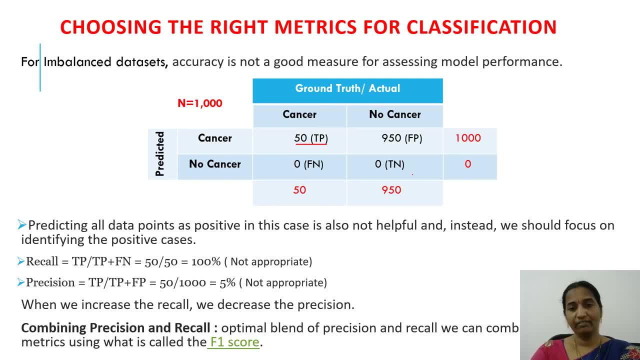 examples are correctly classified as positive and 950 examples are wrongly classified. even then I am getting 100% recall. Now, is it is a good measure? No, Then we can rely on the precision. So precision, if we compute the precision of the value of the model, then it 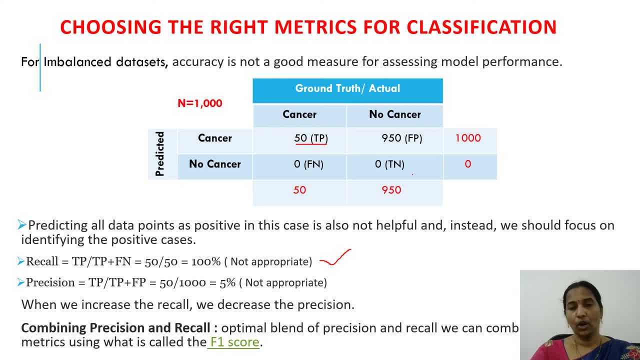 gives the. so what is precision? Precision is how many of the total predicted values of the model are correctly predicted as positive. So that indicates the precision of a model. and when we compute precision it is only 5%. Now we can again understand that the model is not performing. 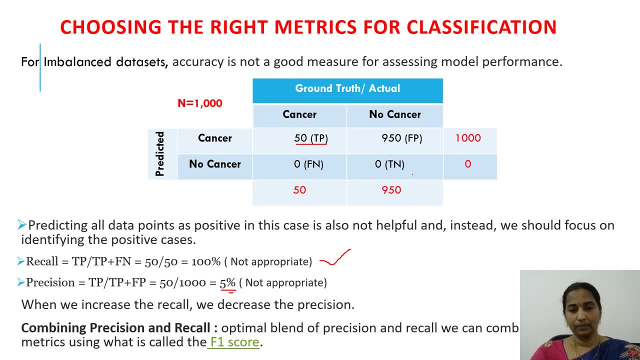 well. So a good indicator of a good performance indicator of the model when the data set is imbalanced, is a F1 score. F1 score is actually a measure that is a combination of precision and recall. So this is how we can choose, depending on the application and depending on the task in. 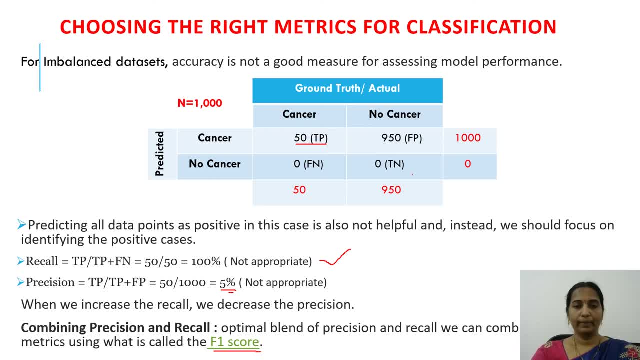 hand, we have to decide which performance, which performance measure, has to be used to measure, to evaluate the performance of the model.